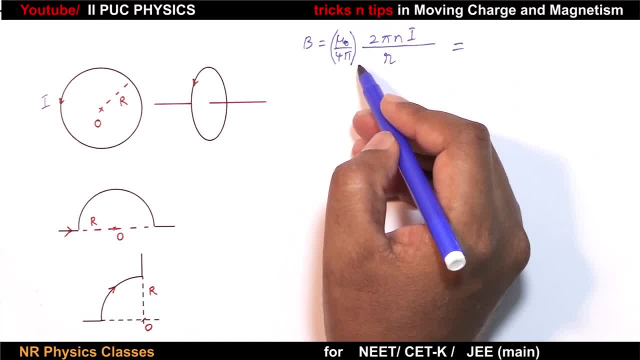 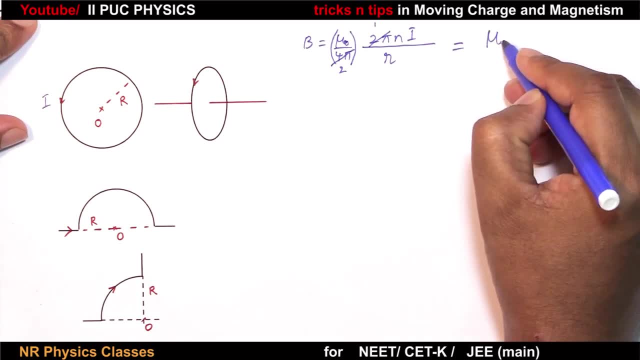 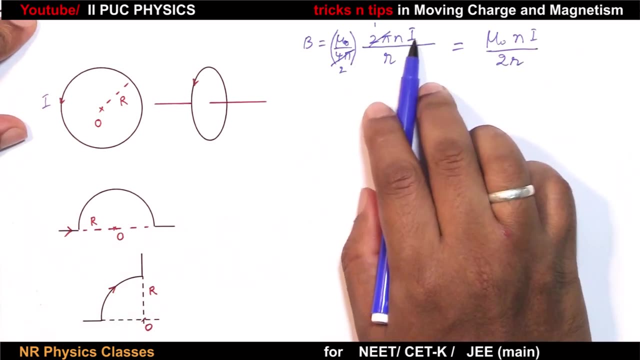 If you simplify this further: 2 pi 1, 2 pi 2.. So this is mu naught n I by 2 R, Constant 2 pi n I by R, Or mu naught n I by 2 R. 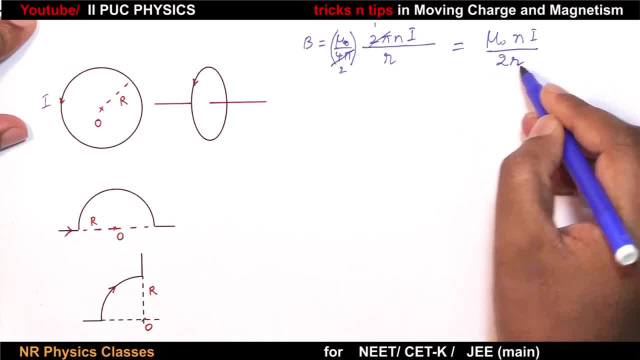 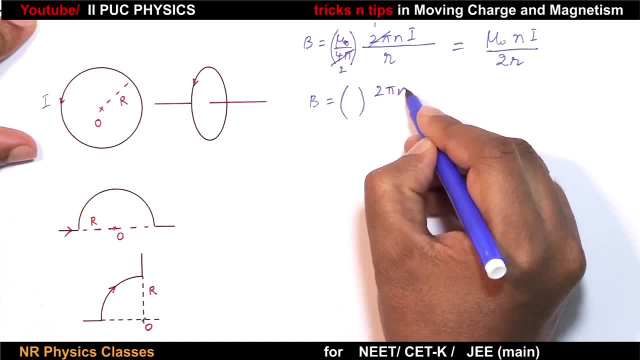 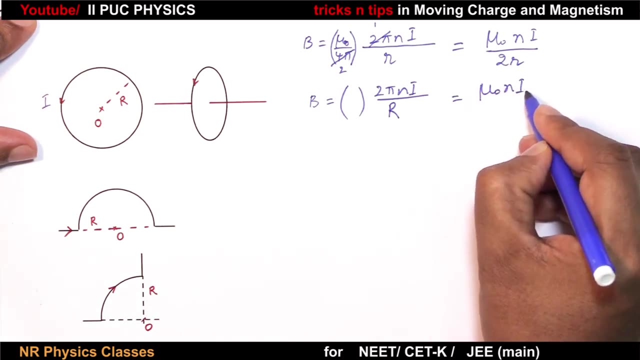 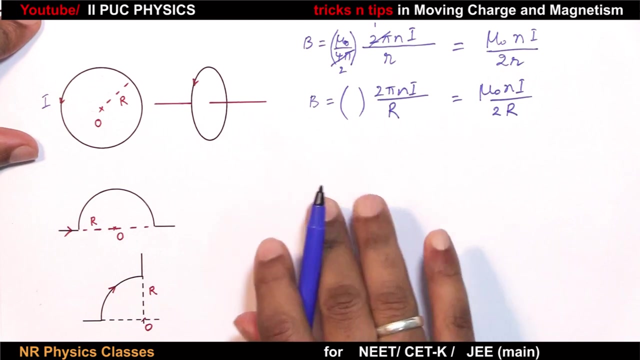 Where n is number of turns in the coil, R is radius, Capital R. Therefore magnetic field is constant: 2 pi n I by R Or mu naught n I by 2 R. Please write and follow all this. Just do not listen and forget. 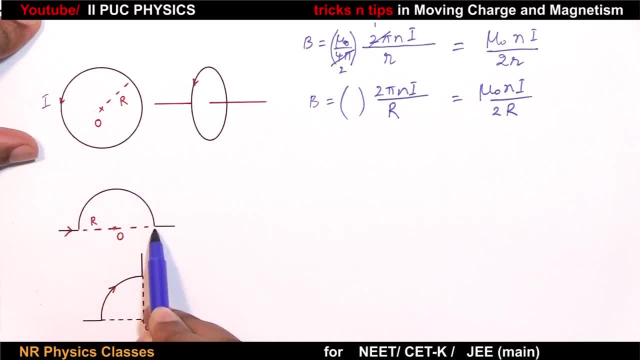 Now second, This is an arc semicircle. If you find straight conductors along the radius, then there is no magnetic field by these straight conductors. Always bear in mind: There is no magnetic field by these straight conductors if they are along the radius. 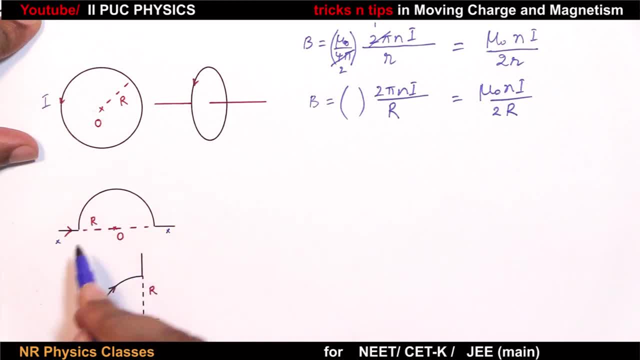 So forget these two conductors. If this is the direction of current, then clockwise it leaves the conductor. Since it is a semicircle, this angle is 180 degree. 180 degree is half of 360.. Nothing, but half of a circle. 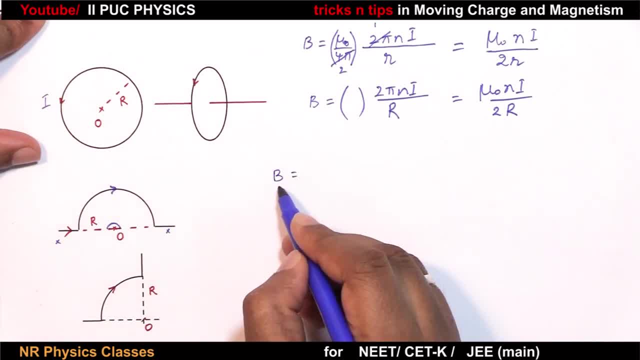 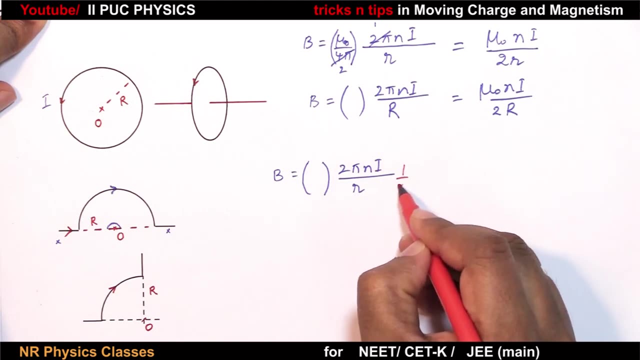 now let me start. first write magnetic field due to circular coil constant 2 pi n i by r, since it is half of a circle, half of this, and this constant is mu naught by 4, pi equal to 2 pi 1, 2 pi 2, mu naught i, mu naught i by 2 into 2, 4 r, 4 radius is r. 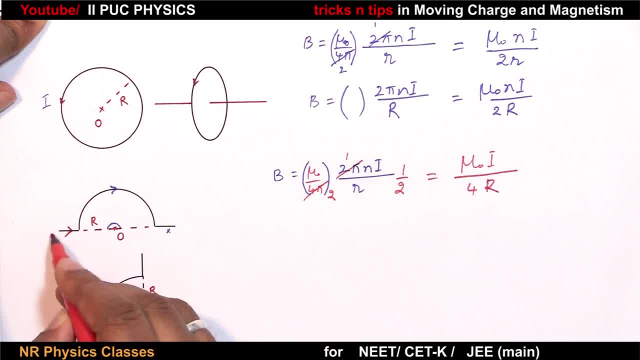 why n is 1 means since a conductor is just bent to form a semicircle. therefore n is equal to 1, so this is the expression. now observe this: these two straight conductors are along the radius, therefore they don't contribute any magnetic field. this arc subtends an angle: 90 degree at the center. 90 degree is 1, 4 of a circle. 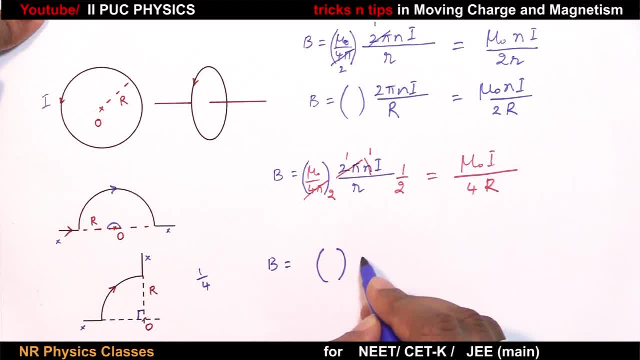 magnetic field due to a circular coil is 2 pi. n. i by r. r is radius constant mu naught by 4 pi. since this arc subtends 90 degree, which is one fourth, this is 1 by 4, equal to substitute n: 1. 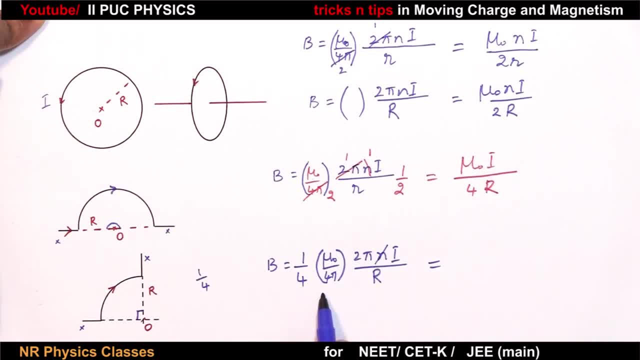 2 pi 1, 2 pi, 2, 4 into 2, 8. denominator is 8 r. numerator is: mu naught i by 8 r, because 2 pi is cancelled with 4 pi 2 times. so mu naught i by 8 r, or else one fourth. 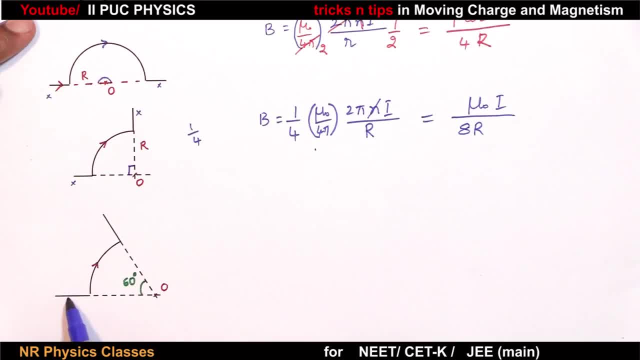 of constant 2, pi, i by r. these two straight conductors are along the radius no magnetic field by the conductors. this arc subtends an angle 60 degree. 60 degree is one sixth of 360.. there, for magnetic field at this point, o is constant 2, pi n i by r, 60 degrees 1, 6. therefore 1, 6. 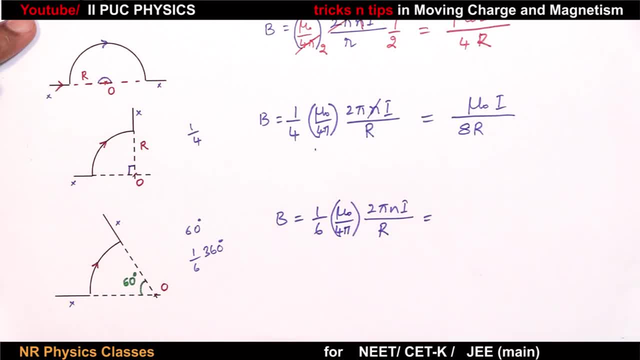 it is mu naught by 4 pi equal. to simplify 2 pi 1, 2 pi, 2, 6 into 2, 12, 12 r denominator is 12 r numerator: mu naught i. i hope it is getting easier now. now observe carefully. there are two arcs. 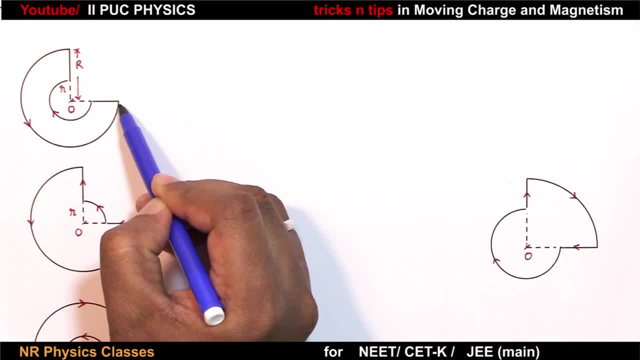 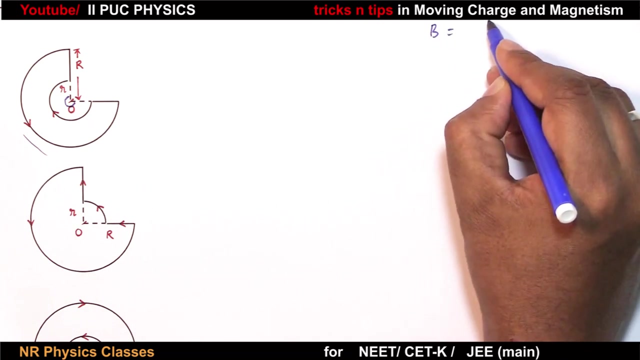 one bigger arc which subtends 270 degree at the center, and a smaller arc of radius. smaller, bigger arc. capital r subtends an angle angle, 270 degree. so let us find the formula first. okay, magnetic field at the center is constant 2 pi n i by r. 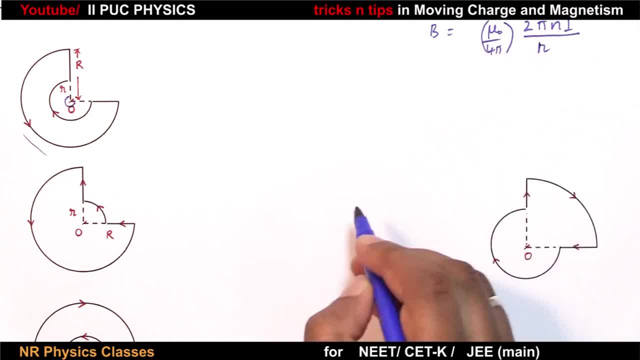 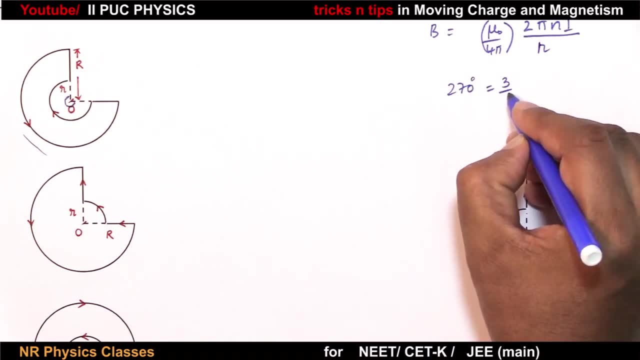 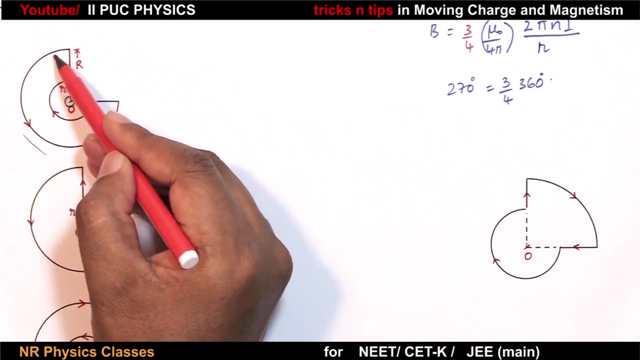 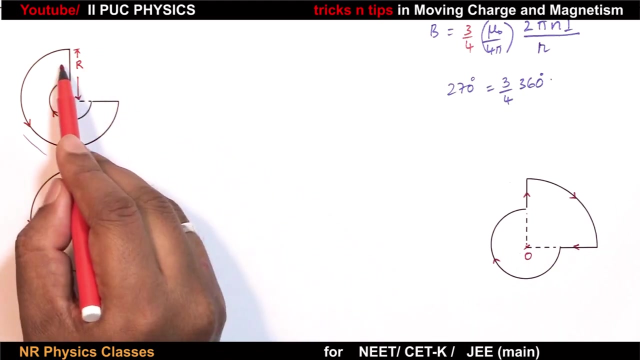 this constant is mu naught by 4 pi, 270 degree. 270 degree is three fourth of 360 degree. so this is md, md, volt quantity. m2 and q is two than cilight without positive hill's, which means that m is three fourth of subtitles together. i am given this الق. 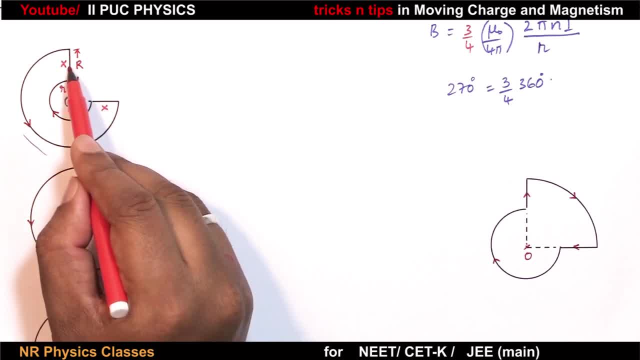 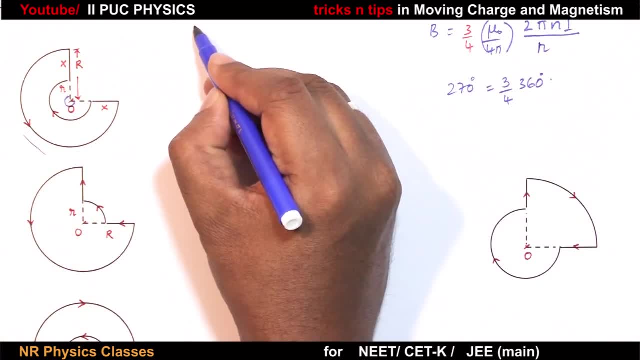 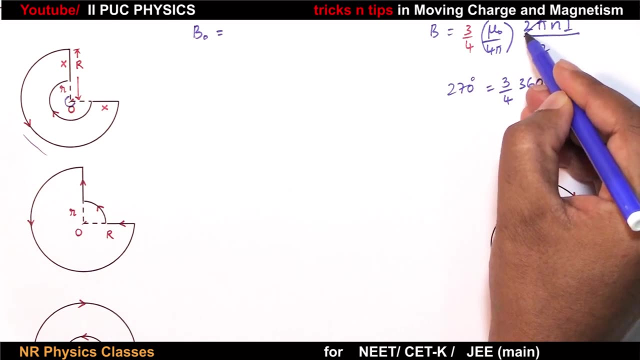 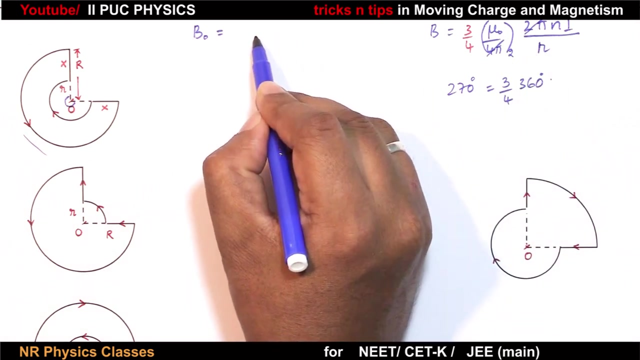 therefore, no magnetic field by these two straight conductors. magnetic field due to outer arc. magnetic field due to outer arc equal, to simplify this, 2 pi 1, 2 pi 2, 4 into 2, 8 r, 8 r. radius of outer coil. 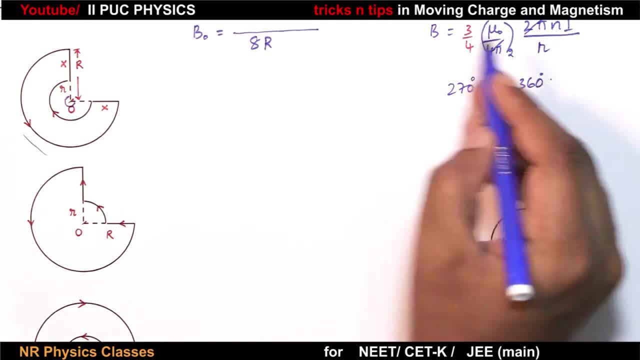 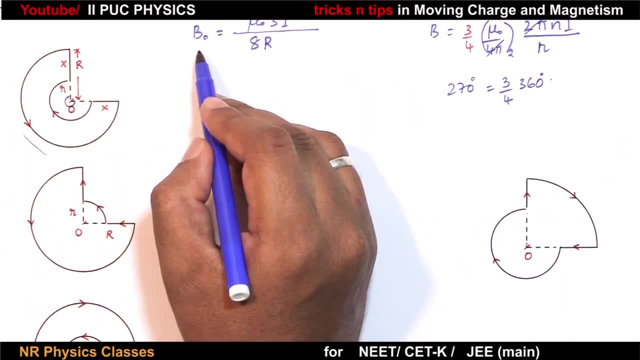 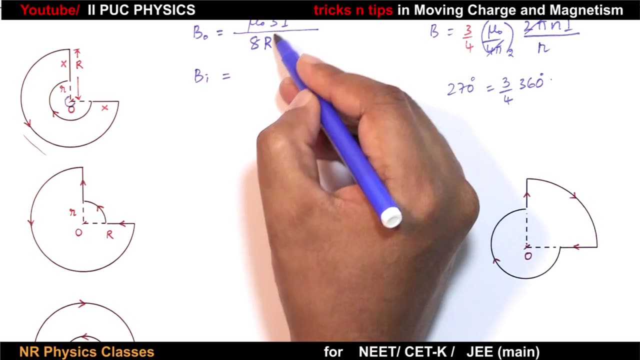 numerator is mu 0 3 i. mu 0 3 i. this is magnetic field due to 3 4th of a circle because of inner arc. magnetic field due to inner is same expression. mu 0 3 i by 8 small r radius. 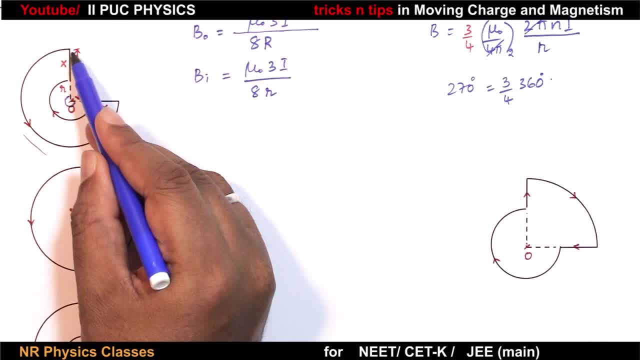 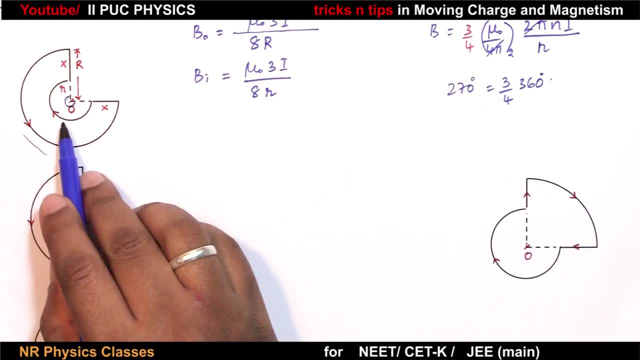 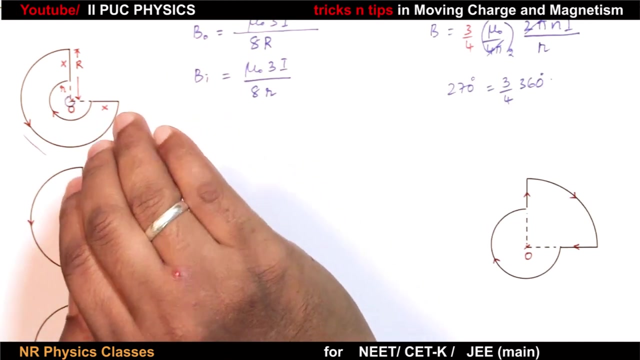 is different. since these two are connected, inner and outer are shorted, so same current flows through them. that is why i and i now magnetic field at the center due to clockwise inner is into the how to find magnetic field due to clockwise current means. keep, keep right hand fingers in the direction of current, open the thumb. thumb gives the. 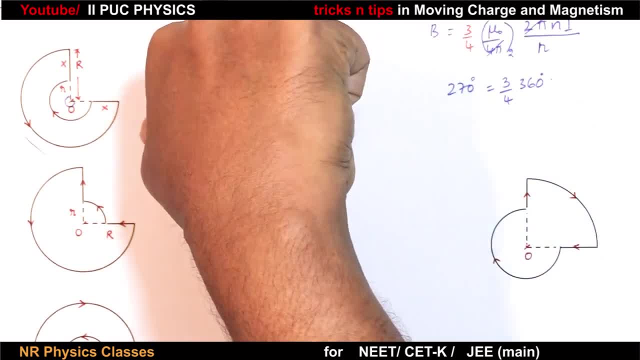 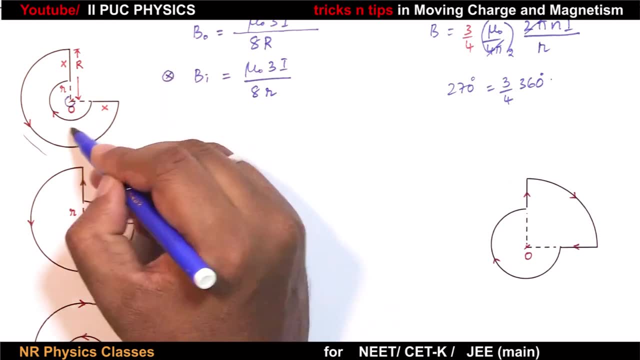 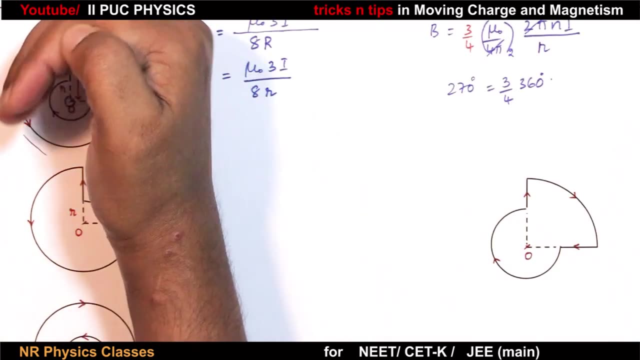 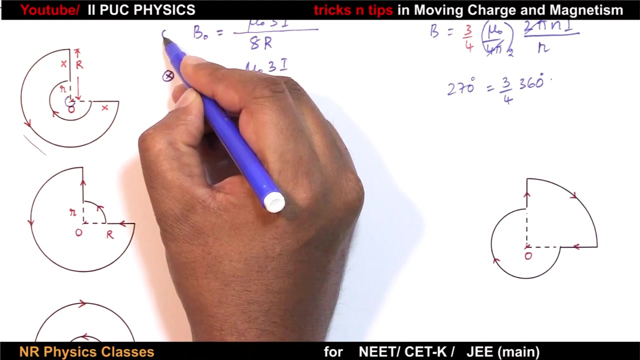 direction of magnetic field. this thumb is perpendicular and into the plane. therefore inner is perpendicular and into the plane, clockwise into, naturally due to outer coil. let fingers be in the direction of current thumb- gives the direction of magnetic field. it is outer. so magnetic field is perpendicular and out. 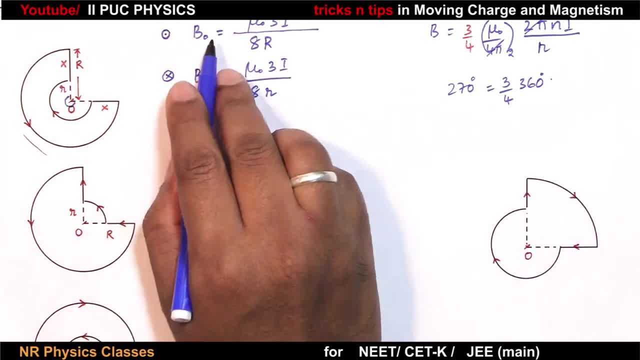 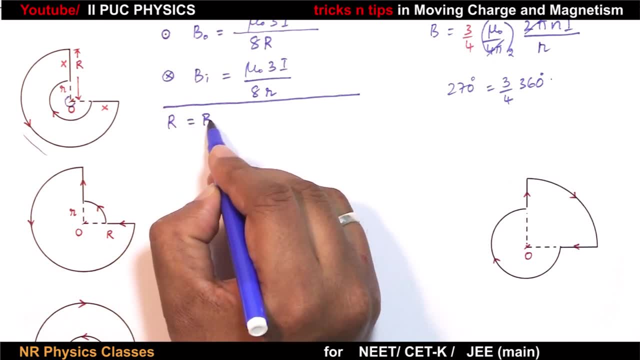 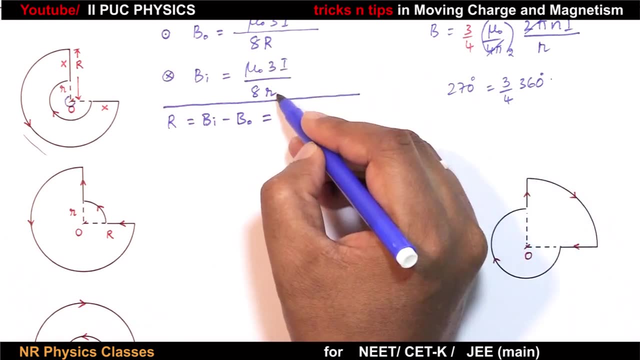 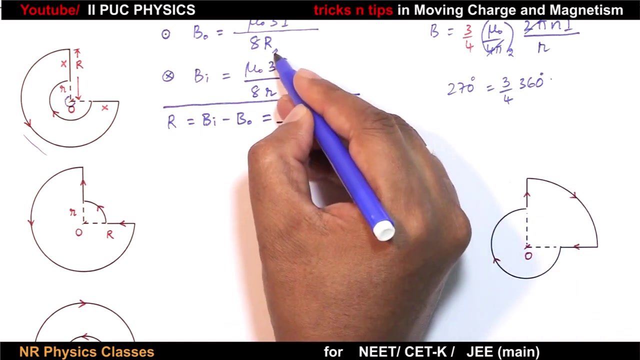 these two are in opposite directions. therefore resultant magnetic field is inner minus outer equal to. in these two, except r, all other terms are common factors. therefore, 3 by 8 mu, 0 i into 1 by small r and minus 1 by capital r. this is the expression. 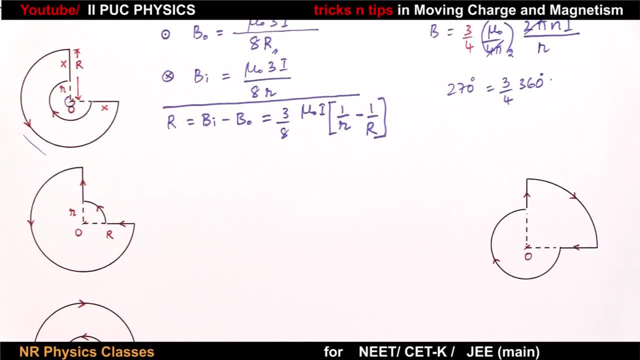 this is the expression Now. in this case it is just three-fourth of an circle. three-fourth of a circle. magnetic field equal to three-fourth of constant 2 pi ni, by radius is r and there is also 90 degree arc. This is magnetic field due to outer, which is equal to 2 pi 1, 2 pi 2, 8,. 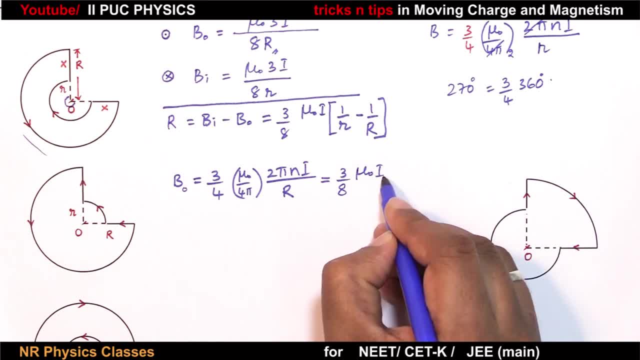 3 by 8.. There is a inner 90 degree inner arc which subtends an angle 90 degree. Therefore, magnetic field due to inner is 90 degree arc. This is magnetic field due to outer which is equal to 2 pi 1, 2 pi 2, 8, 3 by 8.. 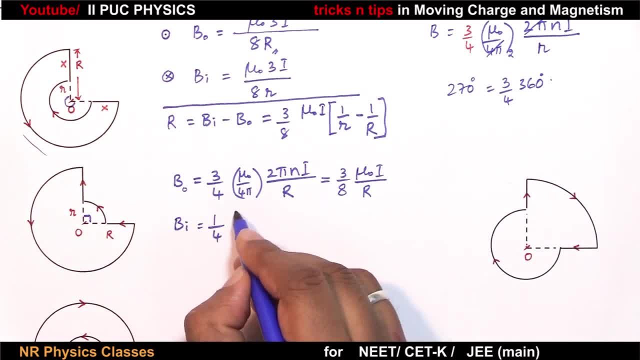 Therefore magnetic field due to inner is one-fourth, One-fourth constant. 2 pi ni by r, r is radius small. r equal to this is mu naught by 4 pi, Again 2 pi 1, 2 pi 2, 4, 2, 8, 8 r. 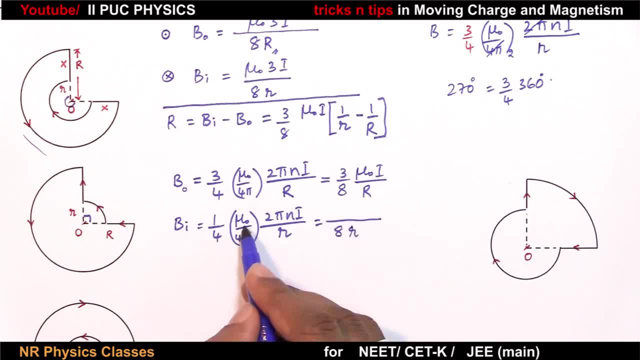 Denominator is 8, small letter r. Numerator is mu naught. i Now observe the direction of current through the outer anti-clockwise, Direction of current through the inner anti-clockwise, So the magnetic fields are in the same direction. 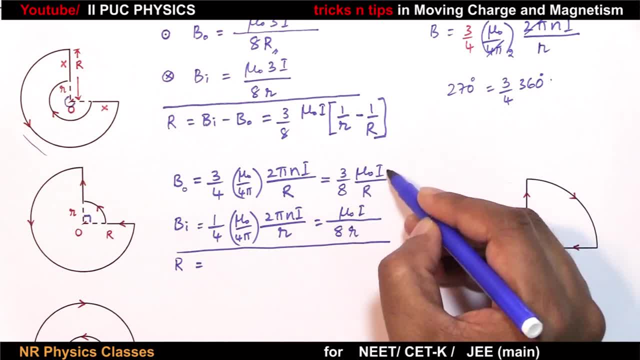 Therefore, resultant magnetic field is sum of these two. In these two, common factor is 3 by 8 mu naught i. Remaining is 3 by 8 mu naught i, 1 by r plus 1 by capital R. 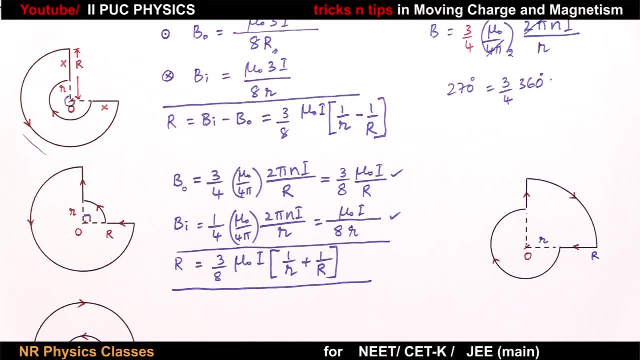 Oh, I made a mistake. Observe 3 by 8,. 1 by 8 is here, So this is 1 by 8.. So there is 3 by capital R, 3 by capital R. This diagram is similar to this diagram. If radius of inner is small r, radius of outer arc is capital R. 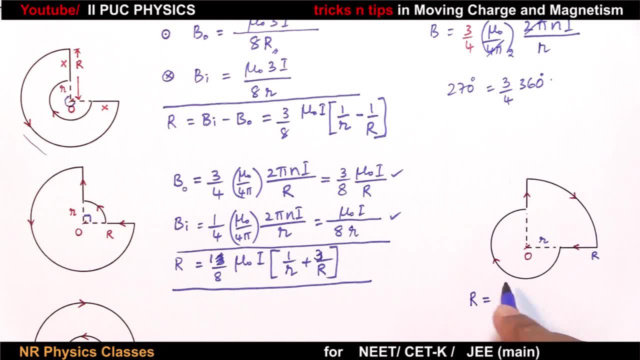 Therefore resultant magnetic field is again mu naught i by 8.. mu naught i by 8 is the common factor Remaining. This is 270.. So 3 by small r plus this is 90 degree 1 by capital R. 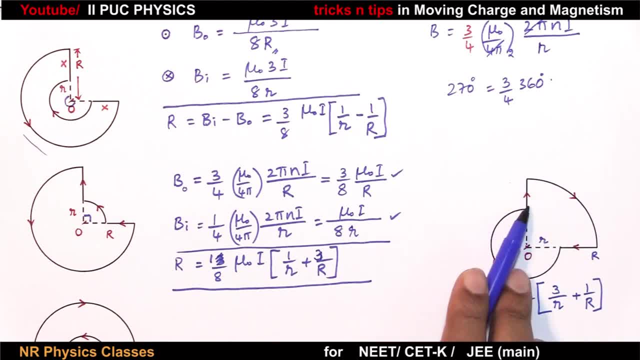 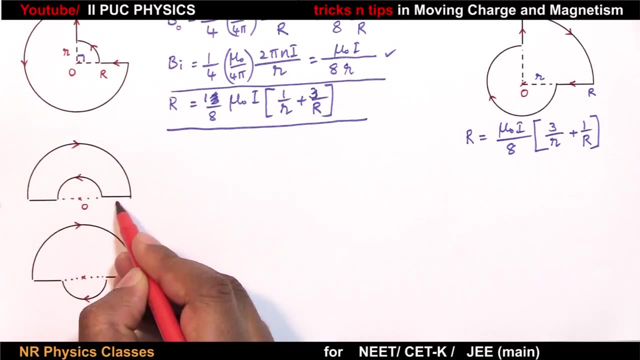 Current through outer is clockwise. current through inner is also clockwise. Therefore, field due to outer is into field due to inner is also into. that results in plus, Semicircle, semicircle. these two conductors are along the radius forget. 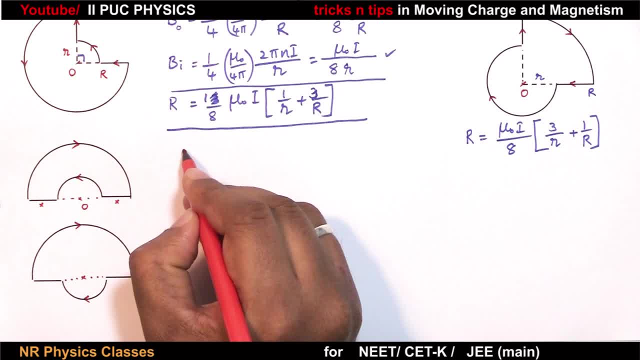 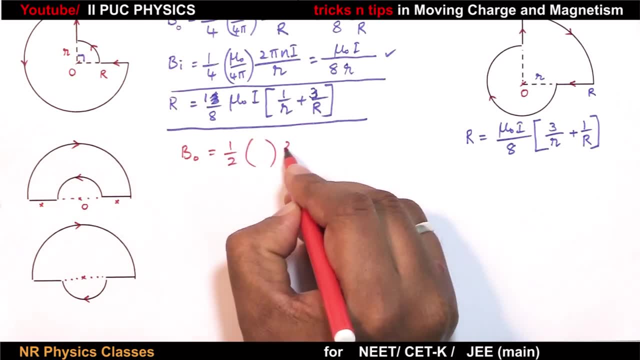 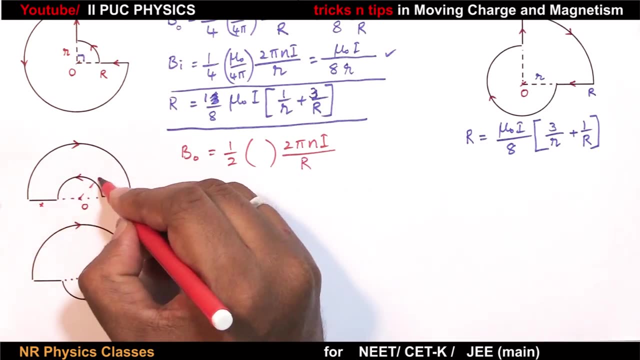 Semicircle. semicircle means half of a circle, So magnetic field due to outer is half constant. 2 pi ni by r r is capital R. let it be capital R. Radius of outer is capital R. radius of inner is small r. 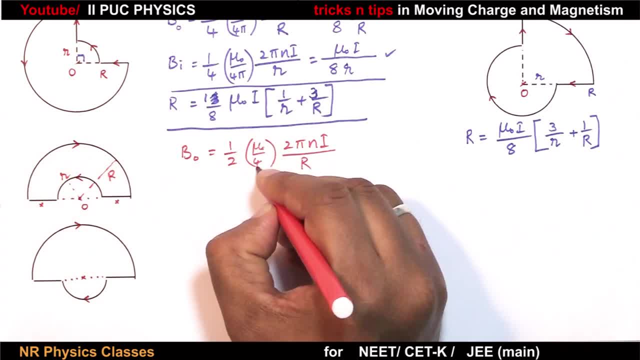 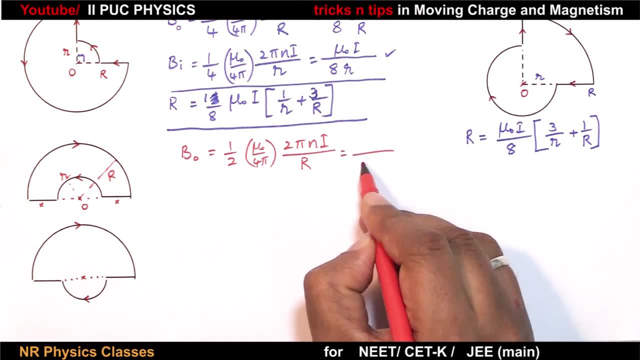 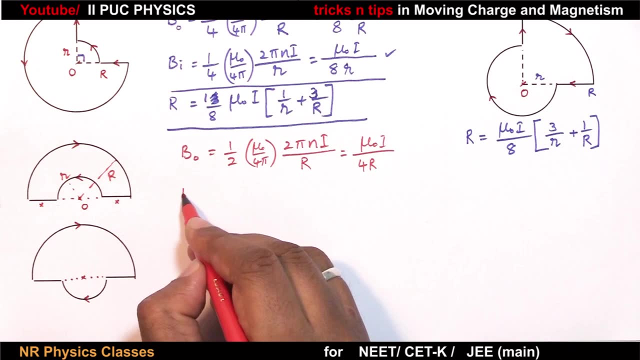 So this is mu 0 by 4 pi 2, pi 2, pi 2 to 4 r. So denominator is 4 r, numerator is mu 0 i, Magnetic field due to inner arc. inner arc is also semicircle. Therefore mu 0 i by 4, small letter r. 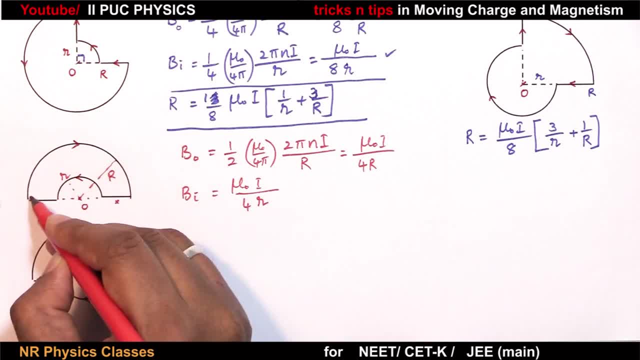 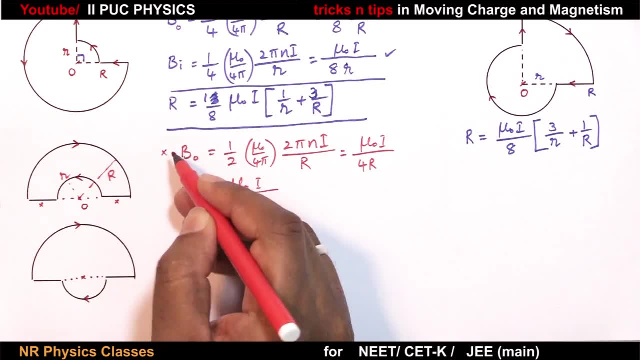 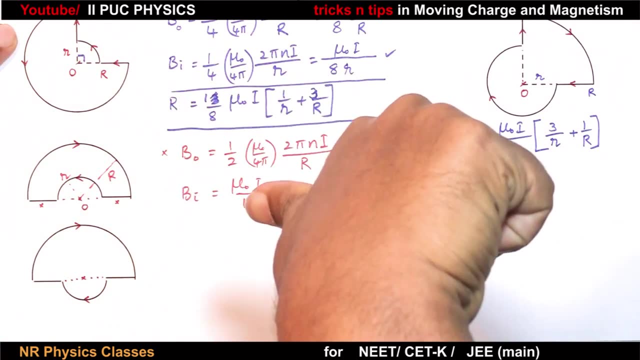 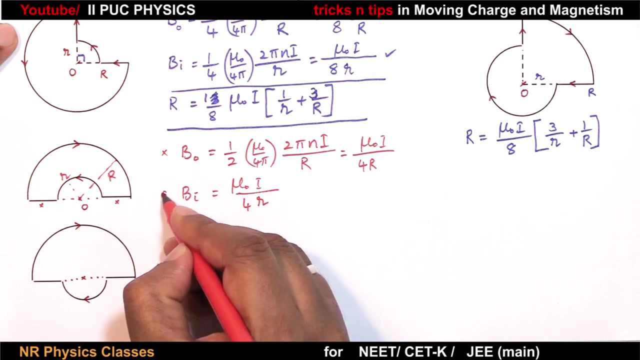 But outer is clockwise. Therefore, field produced by outer at O is into How means Keep curvature of fingers in the direction of current clockwise Thumb gives the direction of magnetic field. Magnetic field, due to inner arc, is outward Perpendicular and outward is represented by this symbol. 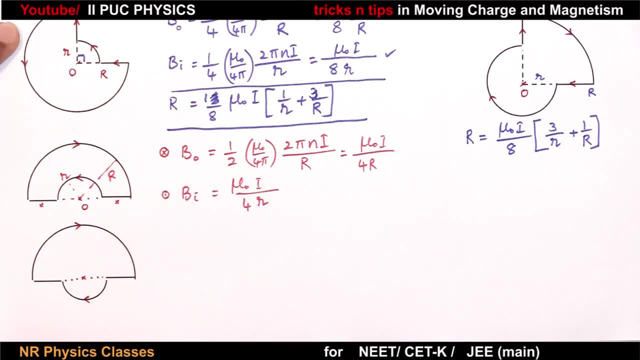 Perpendicular and into Now they are in opposite directions. Therefore resultant magnetic field is common factor is mu 0 i by r, Sorry, mu 0 i by 4, mu 0 i by 4 into 1 by r, 1 by r. 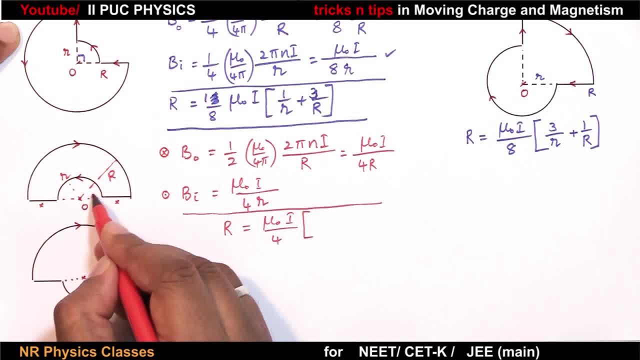 This inner arc is closer to O. Therefore field is more 1 by r minus 1 by Capital r. Consider this Semicircle clockwise, Smaller semicircle clockwise. There is no field due to these two. There is no field due to these two straight conductors. 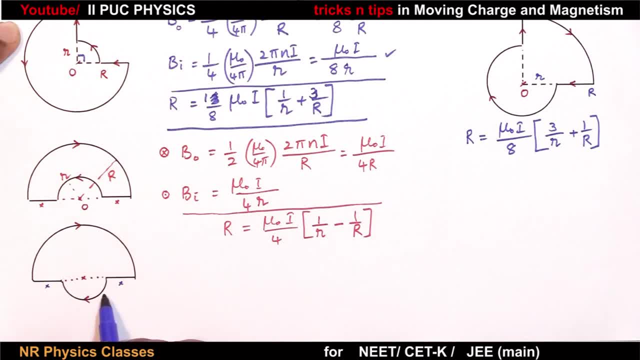 Semicircle clockwise. semicircle, clockwise means. Explanation is similar to this, but with plus, Therefore resultant equal to mu 0 i by 4, 1 by r minus plus 1 by r. Now can we solve a little? 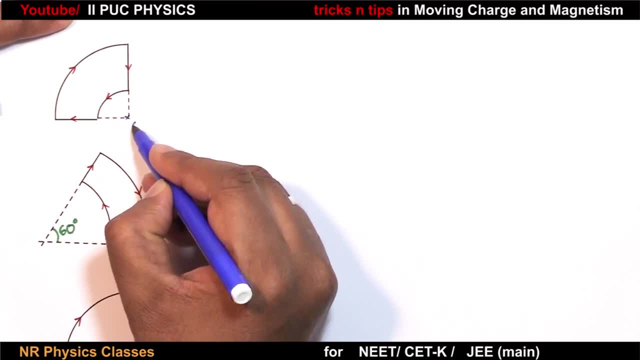 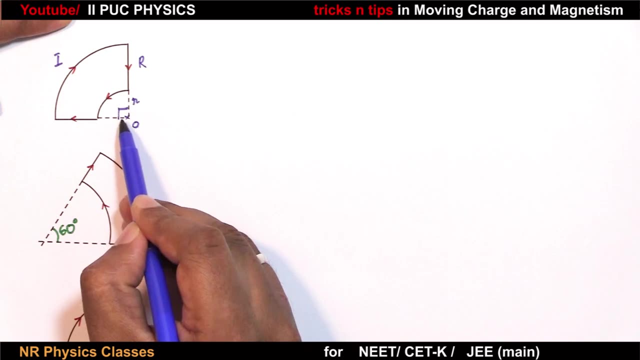 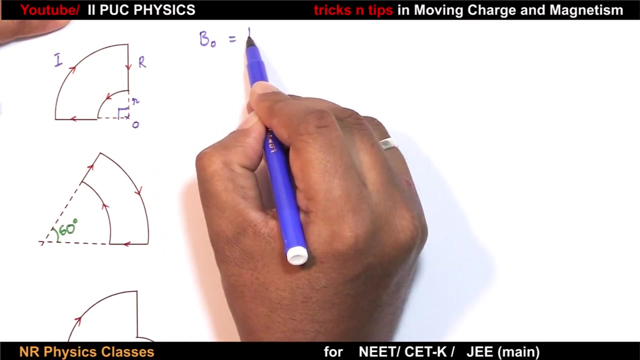 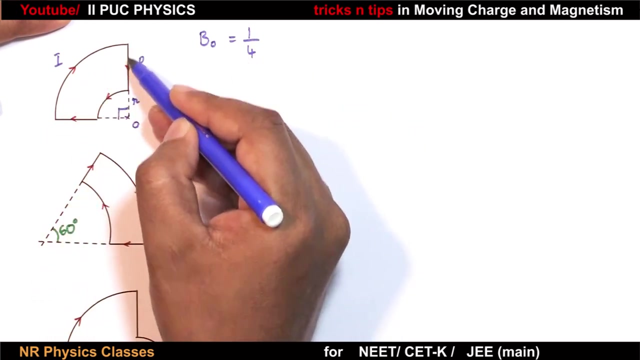 faster. This is O. radius of inner is r. radius of outer is capital R. current is i. This angle is 90 degree. 90 degree means one-fourth Magnetic field due to outer arc is one-fourth of students. why it is one-fourth? Because this arc subtends an angle: 90 degree. 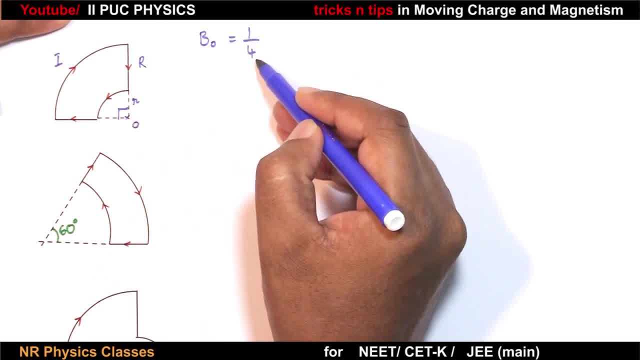 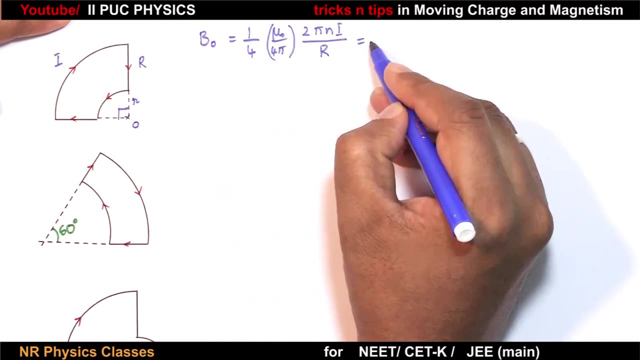 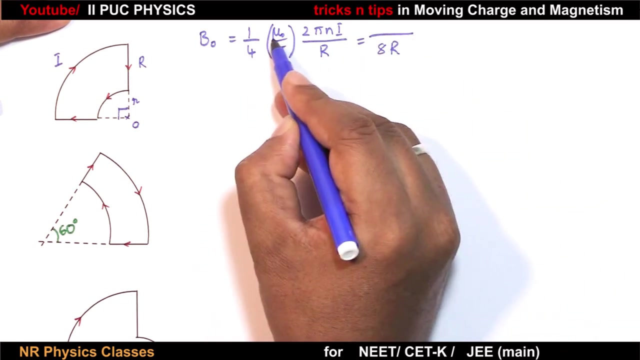 90 is one-fourth of 360.. One-fourth of constant 2 pi ni by r Outer capital R. This is mu 0 by 4 pi Equal to 2 pi 1, 2 pi 2,, 2, 4, 8.. 8 r numerator is mu 0 ni. 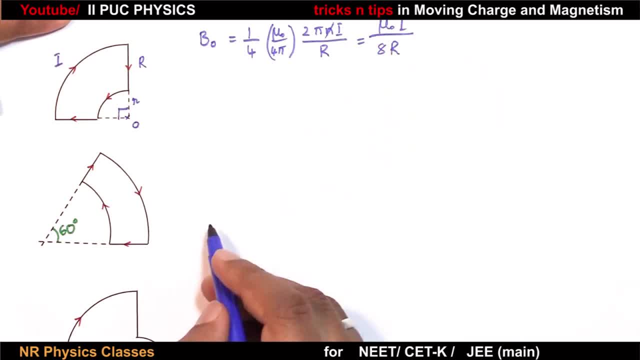 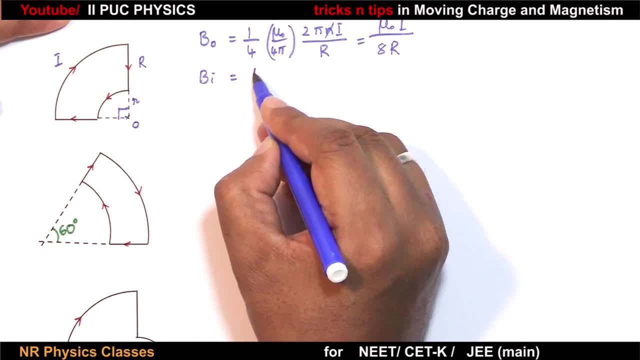 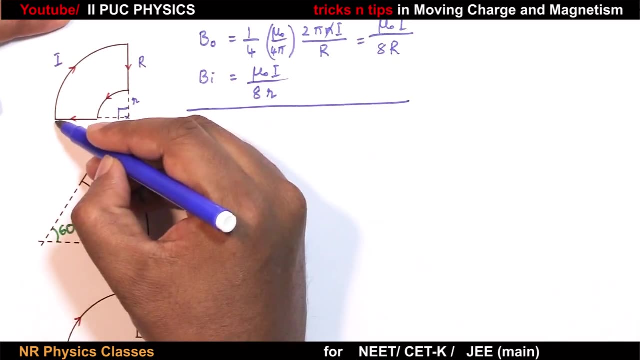 where n is 1.. Mu 0 i. Similarly, magnetic field due to inner is mu 0 i by 8, r, Mu 0 i by 8, small letter r. Outer arc direction of current is clockwise, Inner anticlockwise. Therefore, resultant is: 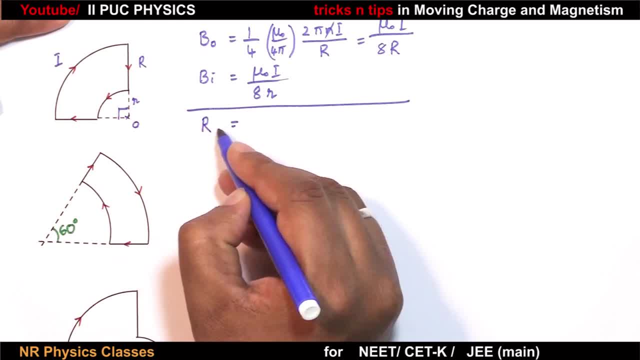 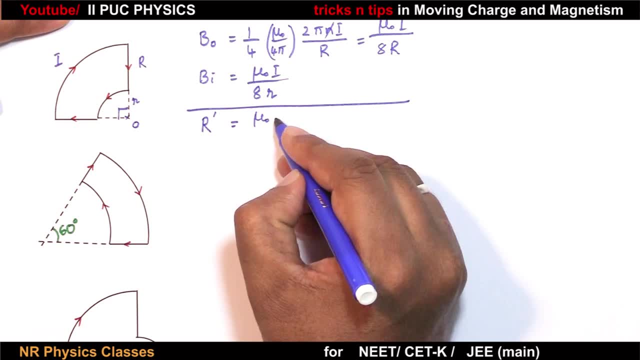 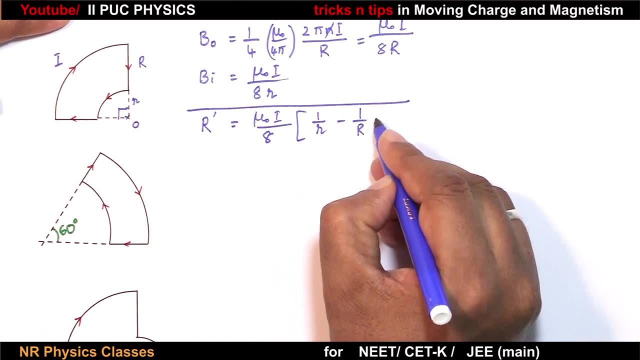 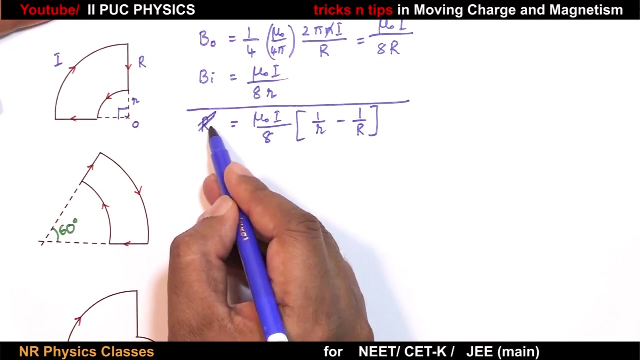 always the difference, Resultant equal to resultant, equal to difference of these two. Common factor is mu 0 i by 8, 1 by r minus 1 by capital. R. R is radius. Since I am using r for resultant, let me denote this by dash, Or else b. b is the. 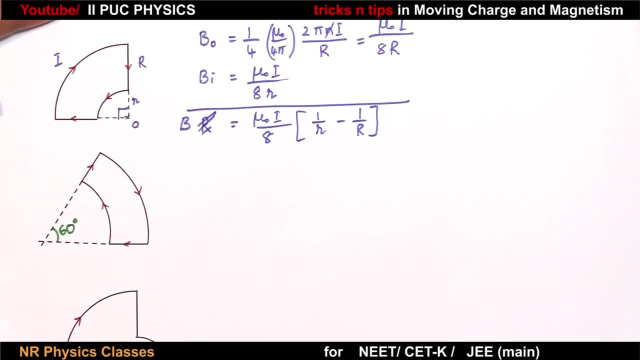 resultant magnetic field. Now observe similar problem, but instead of 90, there is 60.. 60 degree is 60 degree is one-sixth of 360. Therefore, field due to outer is equal to one-sixth of 360.. 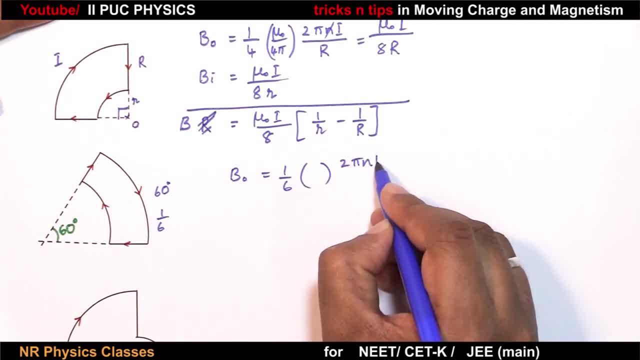 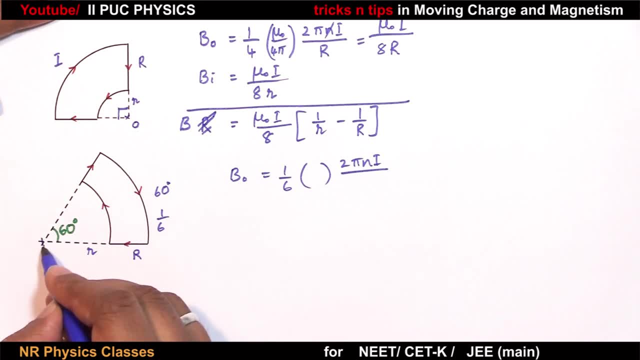 So each of these two cancels off. For example, if there is a constant 2 pi n i by capital r, radius of outer is r, radius of inner is small, r We have to find at more current is 5.. 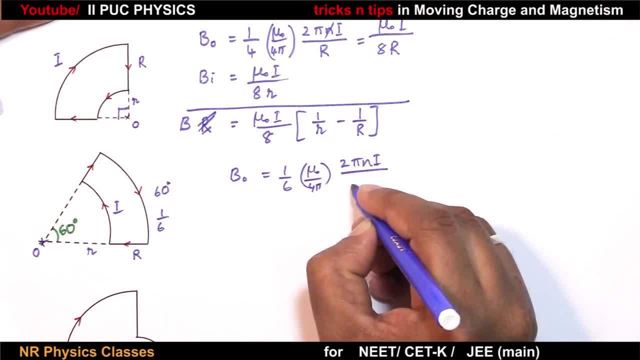 This is mu 0 by 4 pi. Radius is r. Simplify this 2 pi 1, 2 pi 2, 6 into 2, 12, 12. sin R 1 by capital R. Radius is R by capital R Bye. You are acquire raspberry is minus3,j is equal to 4 pi ni by Legend. radius겠지만 a standard radical of that some we have to find. then write to the current current is I, Fine, This is mu. 0 by 4 pi. Radius is r. They say you can use this to find. this seems uy n什么, all right. 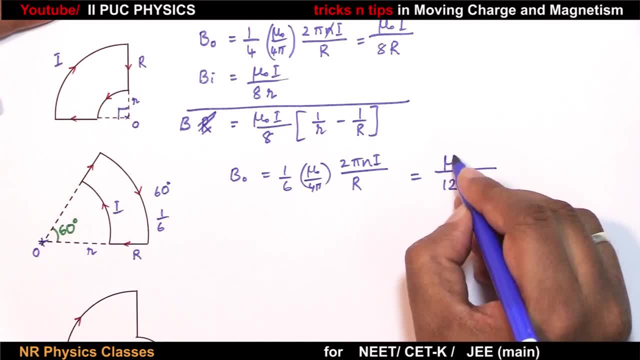 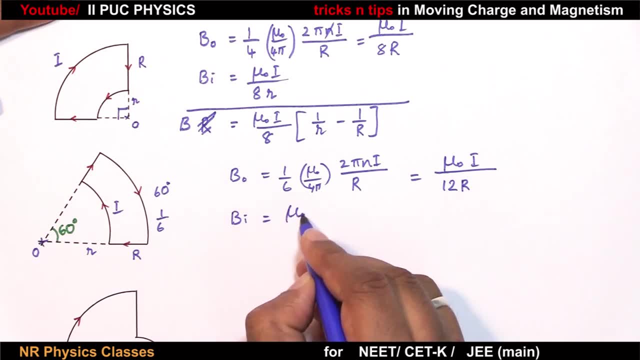 12 r numerator is mu, not i. magnetic field due to inner arc is again mu, not i, by 12 small letter r. radius of inner is small r. okay, one is clockwise, the other one is anti-clockwise. therefore, resultant magnetic field is difference of these two, difference of these two resultant. 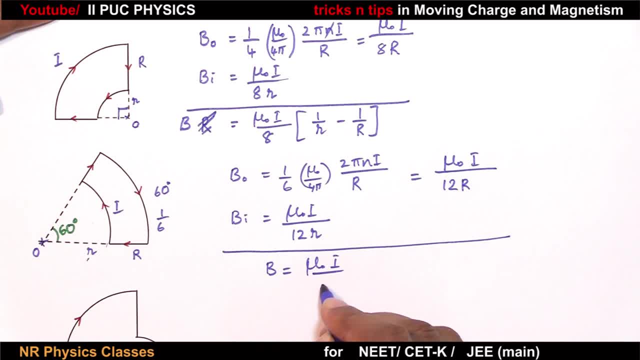 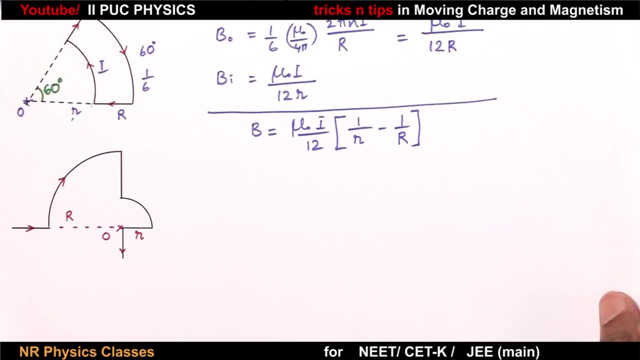 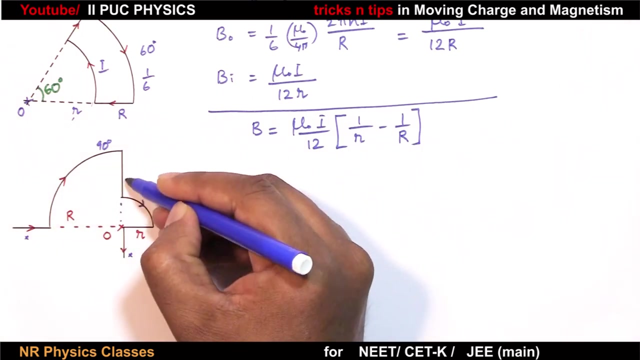 equal to mu, not i by 12. common factor: it is 1 by r minus 1 by capital r. now in this two straight conductors, forget: bigger arc subtends an angle 90 degree. smaller arc also subtends an angle 90 degree. both are clockwise, this straight conductor. 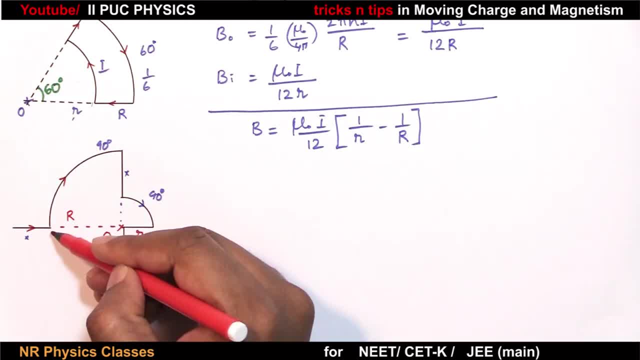 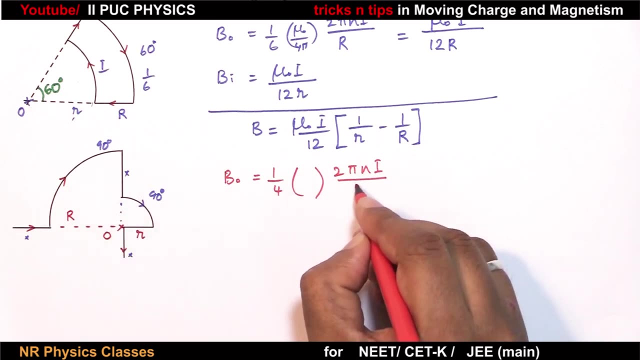 is also along the radius. forget magnetic field due to outer arc. one-fourth. one-fourth is because of 90 degree one-fourth constant 2 pi n i by radius. is capital r equal to 1 by 1, 2 pi n i by 2, pi 1, 2, pi 2, 4, 2, 8. denominators, 8 r numerators, mu not i. 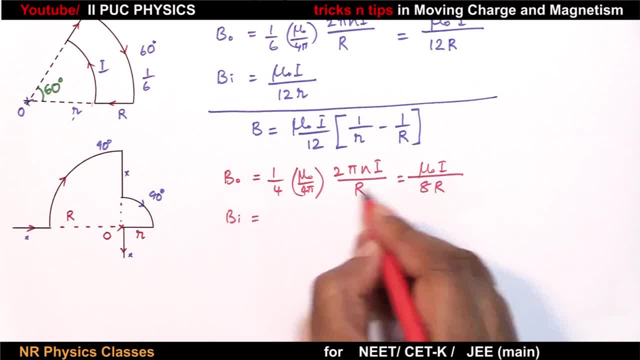 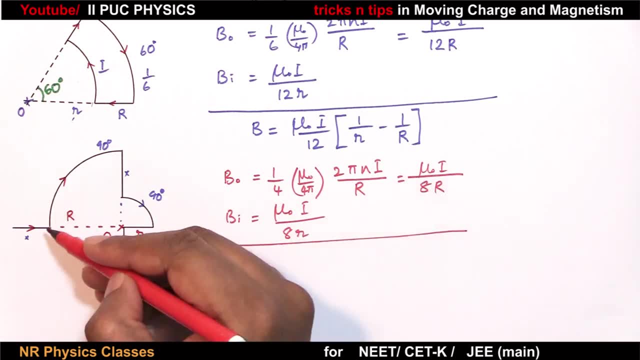 now, magnetic field you to inner arc is same thing, 8 smaller. so resultant of these two means clockwise magnetic field is into anti-clockwise magnetic field is into. therefore resultant field is sum of these two. mu naught I by 8 into 1 by R plus 1 by capital R, some. 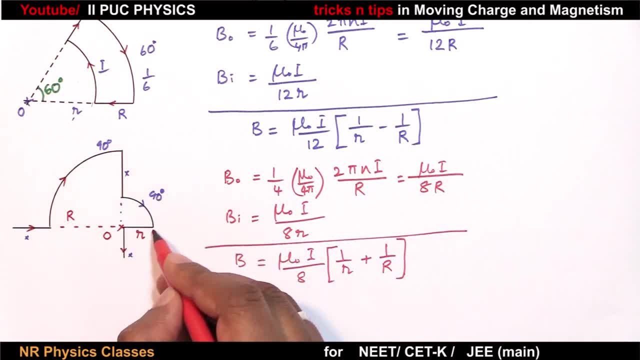 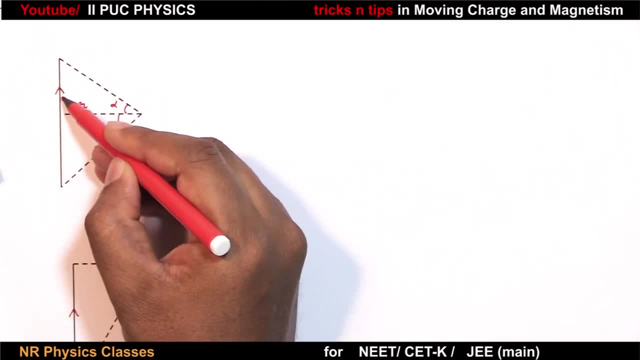 because directions of currents are same. directions of magnetic field is also same. this is little different. straight conductor direction of current is upward R and current is I at O. we have to find magnetic field. magnetic field at some point due to straight conductor carrying current from ends of the. 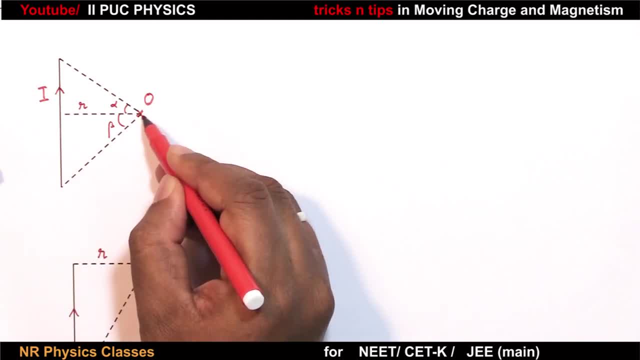 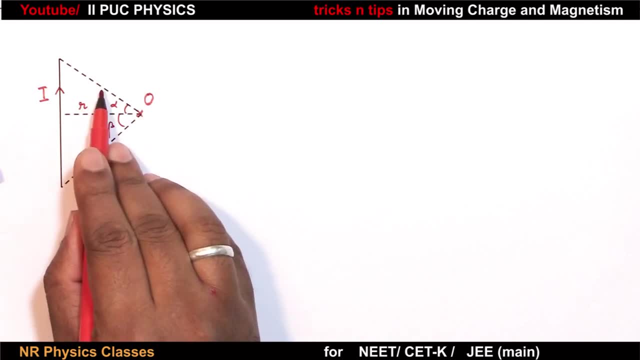 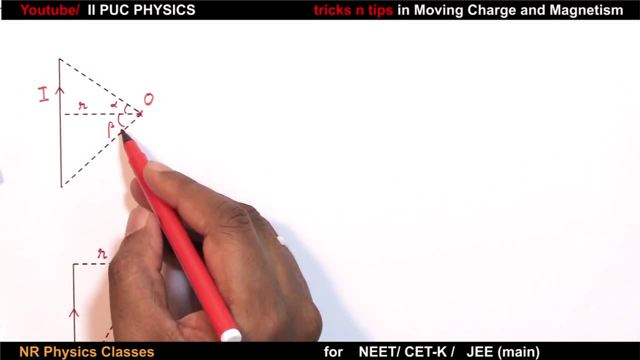 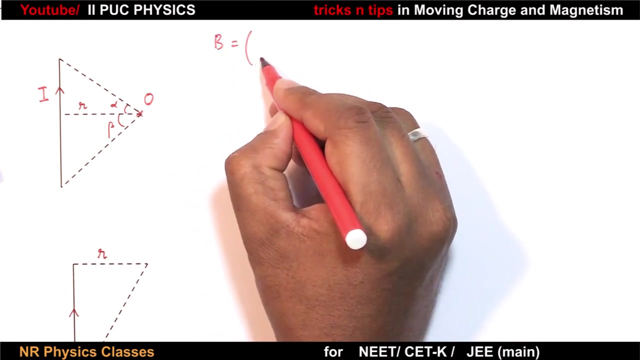 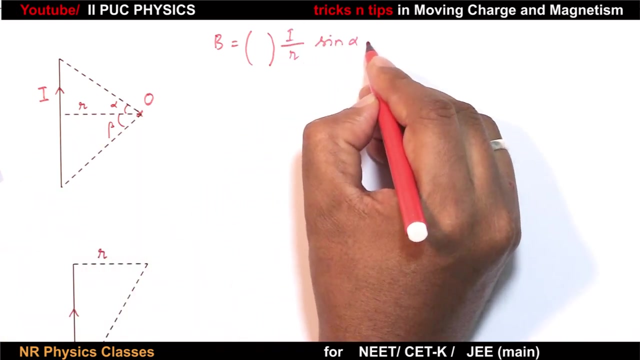 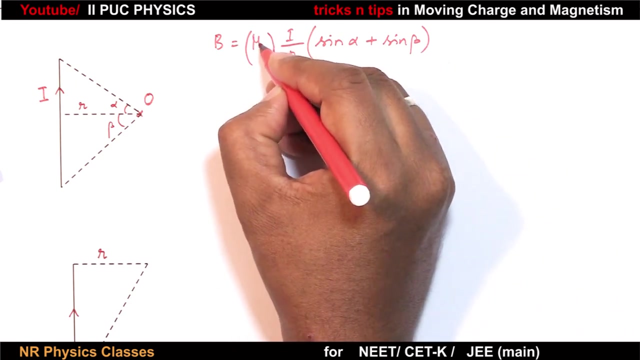 conductor draw lines to the point these two dotted lines. shortest distance is R angle between this line and the shortest distance alpha from the other end. beta magnetic field at O, due to current I, is magnetic field equal to constant I by R sine alpha plus sine beta. this is the general equation. this constant is mu. 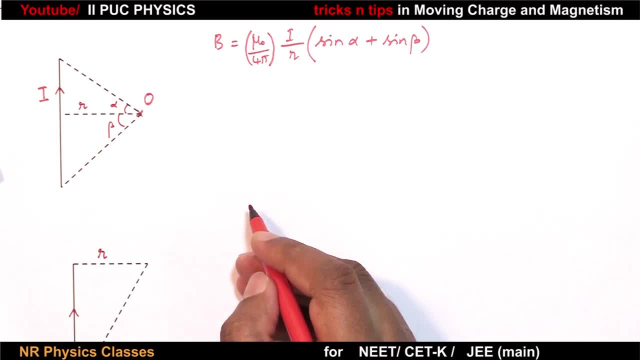 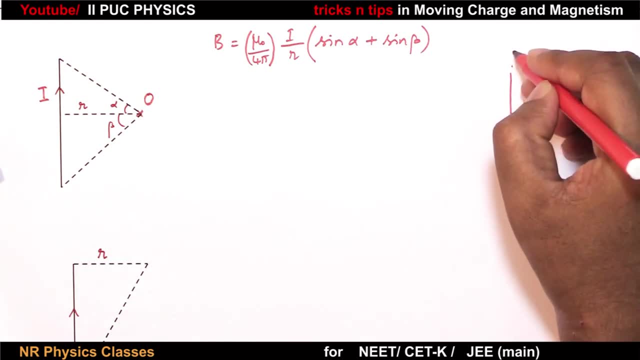 naught by 4 PI. ok, fine, suppose if there is a conductor of infinite length. conductor of infinite length means on either side we can find conductor, and this is point o. from that infinite end to o i have to join by dotted line. this is the shortest. 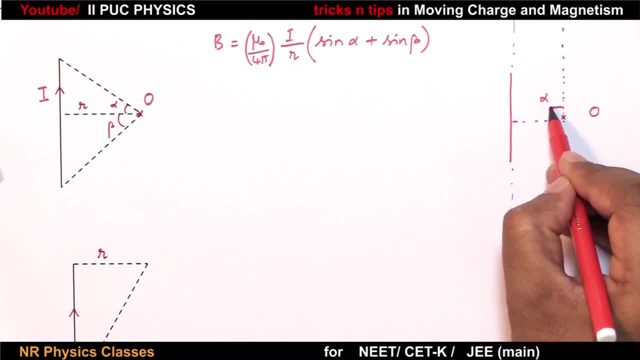 distance alpha is 90, almost 90. conductor is of infinite length, so from point o to that lower end i have to join by this dotted line. this beta is also 90. therefore, if there is a straight conductor carrying current of infinite length, then magnetic field at some point is given by 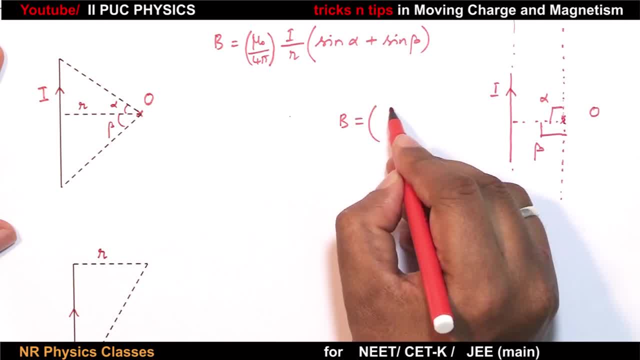 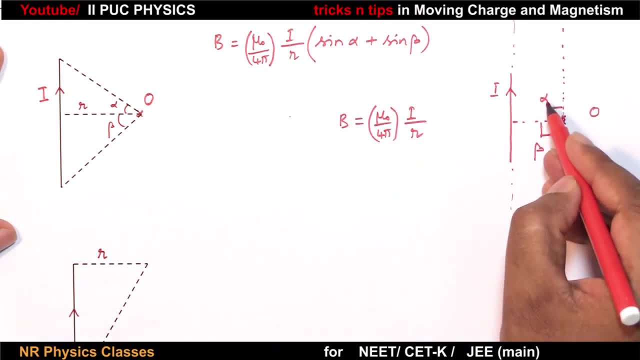 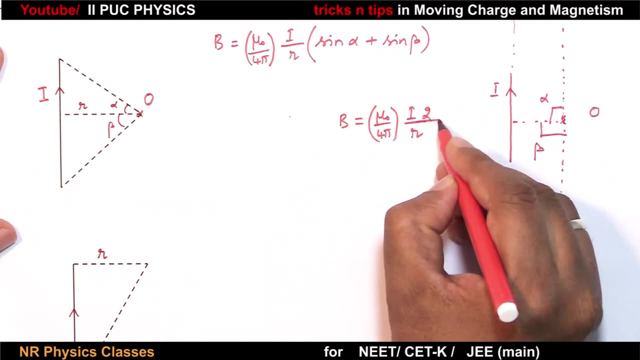 b equal to constant mu naught by 4. pi i by r sine 90 sine 90.. sine 90 is 1, 1 plus 1 is 2.. so it is 2 i by r. this equation we have derived from ampere circuit law. this is there in our syllabus right. constant 2i by r. this equation is only for. 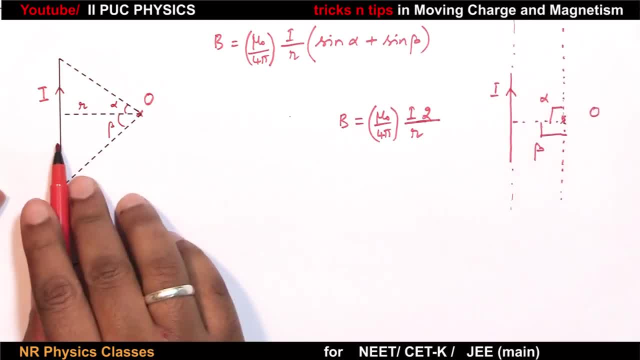 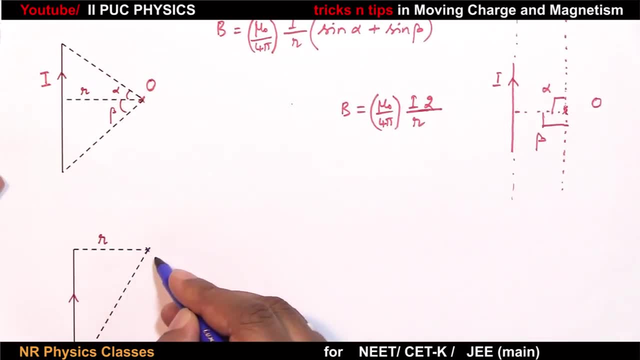 straight conductor of infinite length. this is for finite length. okay, one more special case. what if the point is at one end of a straight conductor of infinite length? infinite length, infinity. it is going down. this is one end of the straight conductor. r is shortest distance. this dotted line from this end, let me draw. 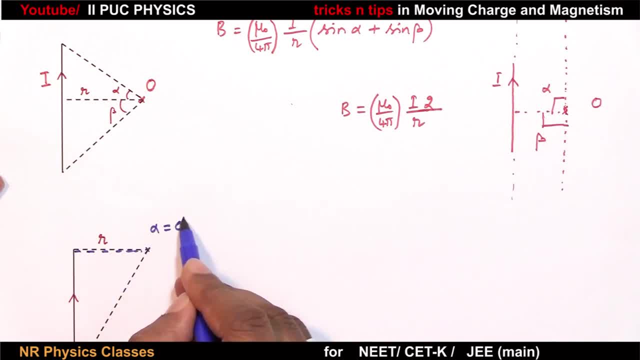 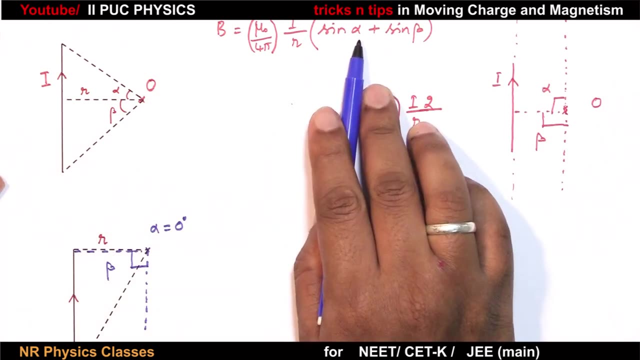 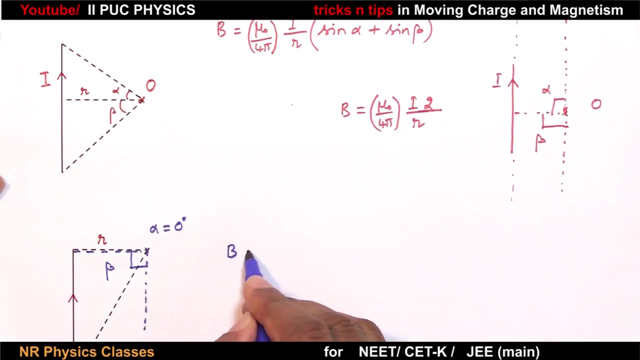 a dotted line, so here alpha equal to zero. if the conductor is of infinite length, then naturally i should draw this line, and this turns out to be beta, and beta is 90.. sin 0, sin 90, sin 0 is 0, sin 90 is 1. therefore, magnetic field at one end of the conductor is: 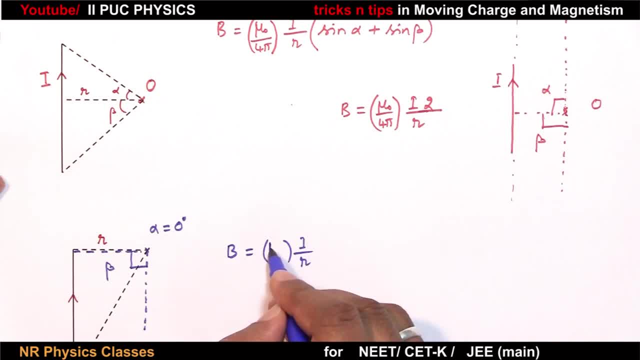 constant i by r, mu naught by 4 pi. see if this is a straight conductor of infinite length. direction of current is i. magnetic field at any point is constant 2 i by r. magnetic field at one end of the conductor is constant i by r, 2, i by r. i by r. observe this diagram carefully. current is i. 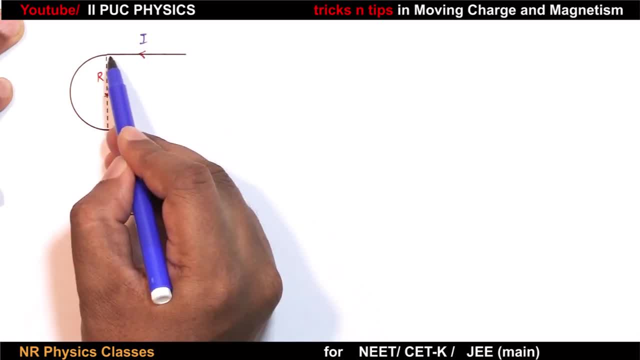 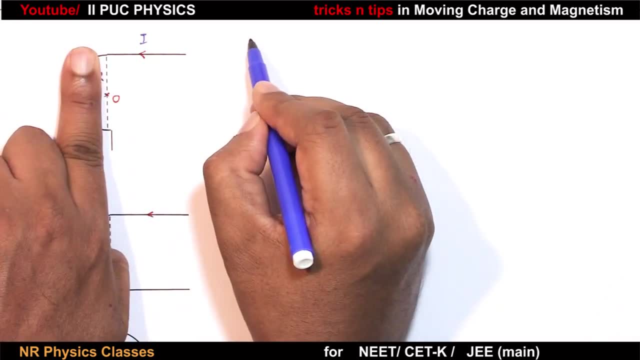 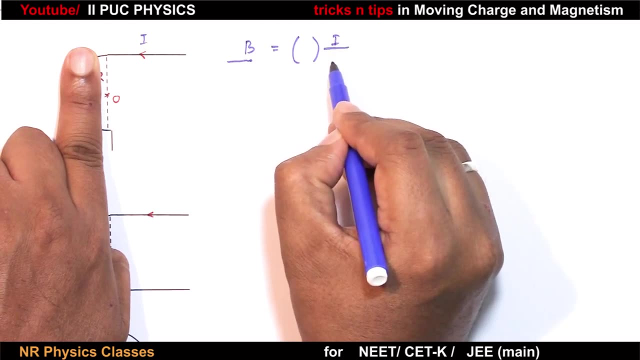 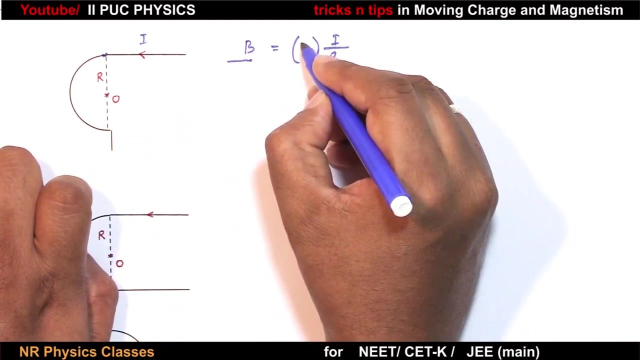 there is a straight conductor and point is at one end of the straight conductor, see conductor, one end. so magnetic field due to one end of a straight conductor is constant i by r, where r is distance between conductor, and o, which is equal to radius. r constant is mu naught by 4 pi. 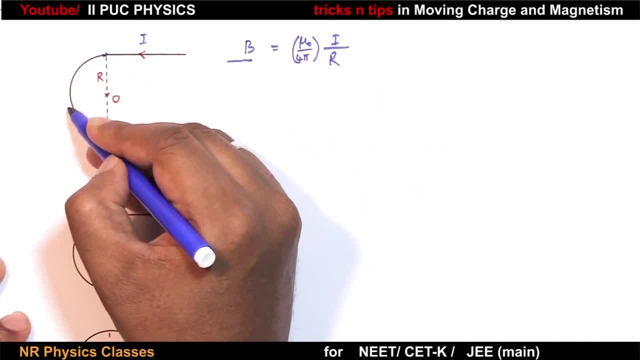 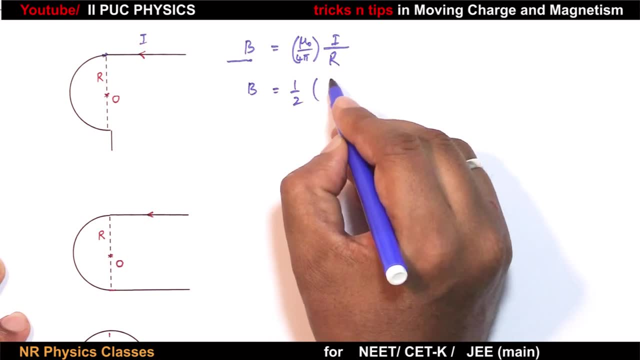 now there is an arc semicircle, so magnetic field due to semicircle is half constant. 2 pi n i by r, which is equal to this, is mu naught by 4 pi 2, pi 1, 2, pi 2, 2, 2, 4, 4 r. denominator is 4 r. 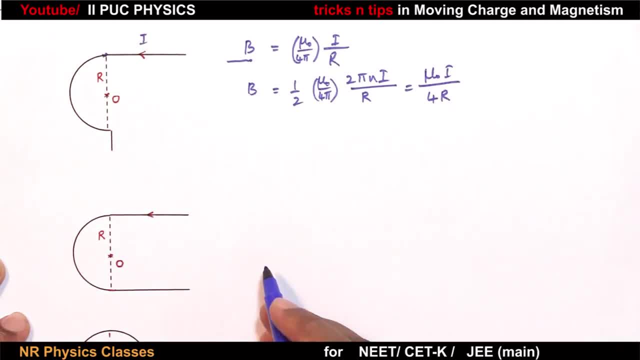 numerator is mu naught i. so this is magnetic field due to semicircle, magnetic field due to straight conductor. this straight conductor is along the radius. therefore this won't contribute to the magnetic field. now, if this is the current, current through the arc is anticlopwise. 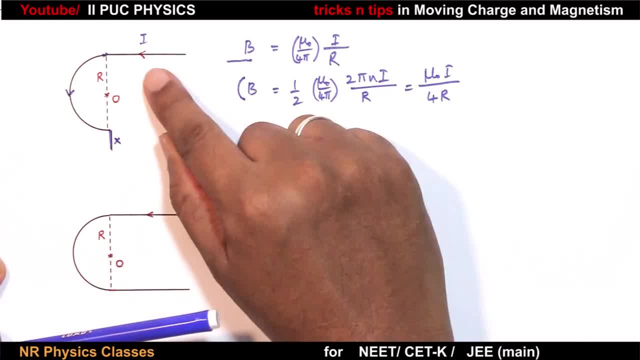 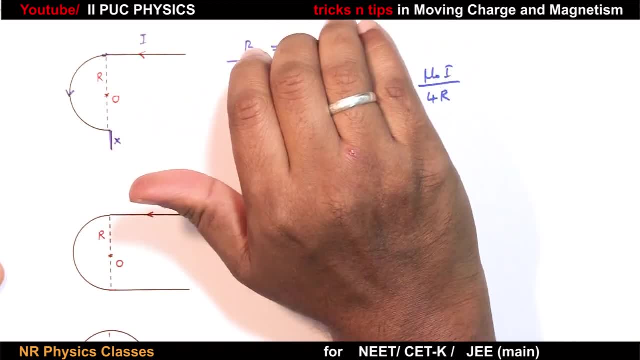 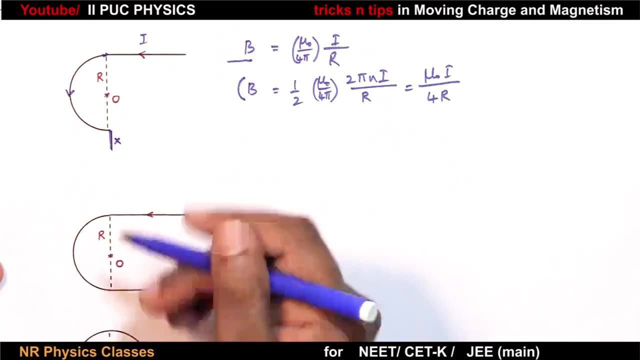 for straight conductor, use right hand clasp rule. if thumb is imagined to be in the direction of current, then curvature of fingers gives the direction of magnetic field. okay, like this at o: magnetic field is perpendicular and outward. due to this, i straight conductor, is primeiro, and Hero believed in this idea. now let's look further at the어 quintessentialing for the curve n. 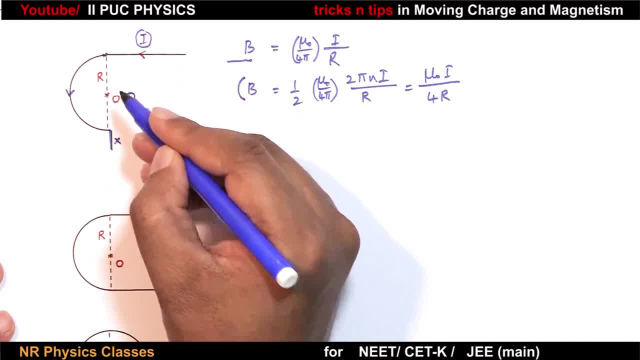 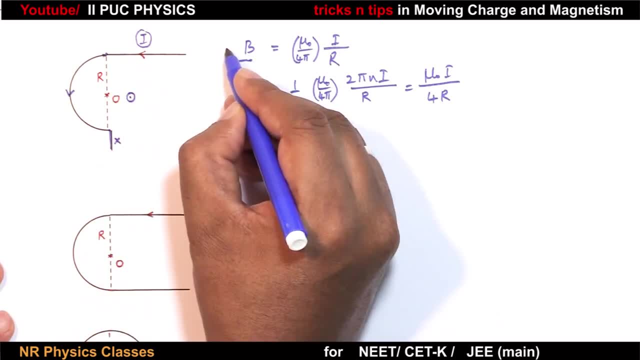 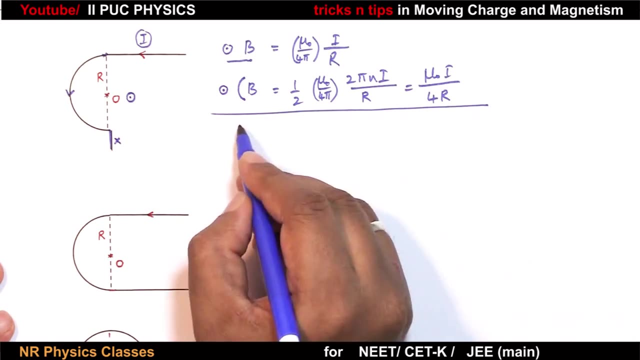 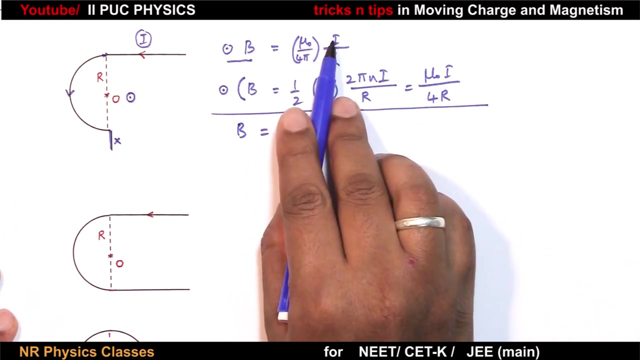 and i by p nada conductor magnetic field is outward. if it is anti-clockwise magnetic field is outward. therefore this magnetic field is outward, this magnetic field is also outward. so resultant magnetic field equal to sum of these two. observe in these two: mu 0 i by 4 r, mu 0 i by. 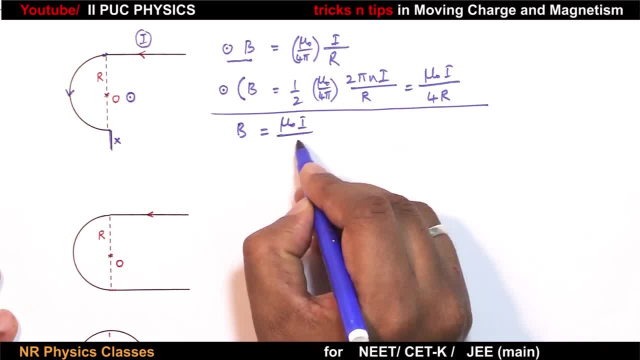 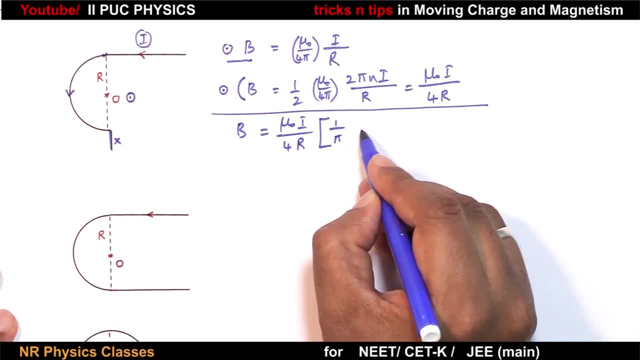 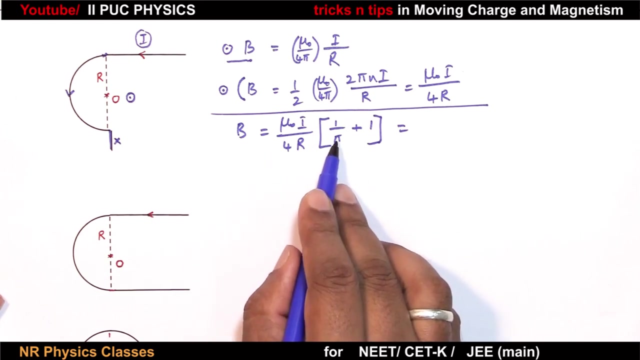 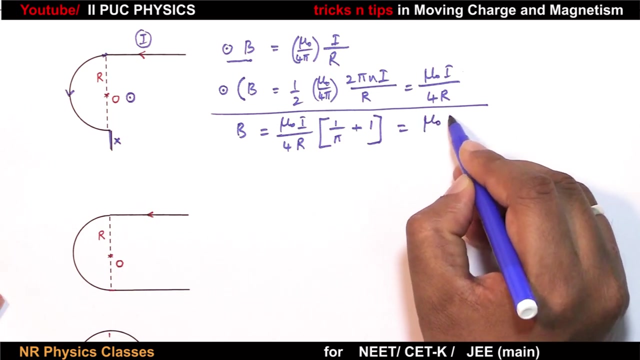 4 r. common factor: mu 0 i by 4 r. remaining is 1 by pi plus 1 equal to. in multiple choice questions we can also find the simplified form. one more form: take pi outside. take pi outside. mu 0 i by 4 pi r into pi is outside means. 1 plus pi by pi. denominator pi is outside means. 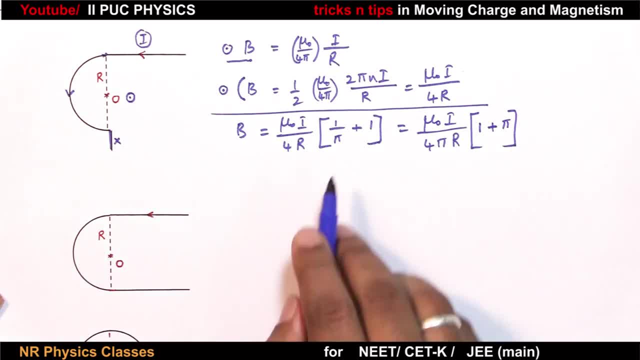 there should be a numerator pi. you can find answer in this form or in this form now, little faster: stride conductor. this o is at one end of the conductor. therefore, magnetic field due to stride conductor. magnetic field at one end due to stride conductor. constant i by r. 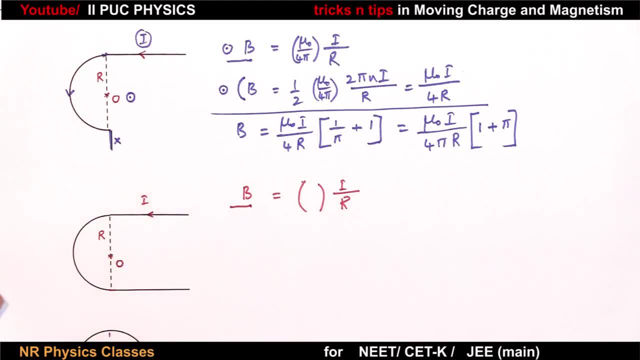 radius is the shortest distance. now, semicircle magnetic field due to semicircle is constant, half constant: 2 pi n i by r 2 pi 1, 2, pi 2, 2, 2, 4, 4 r, mu 0 i now because of this stride conductor. observe, these two stride conductors are not along the radius. 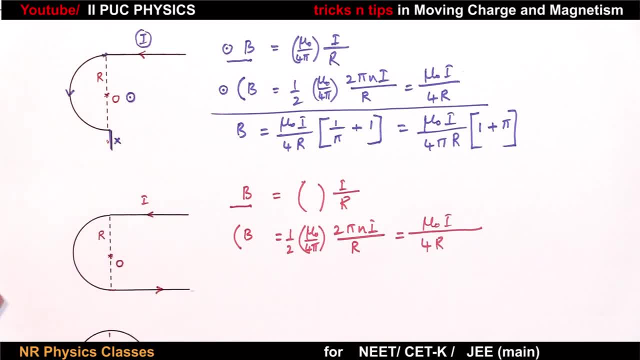 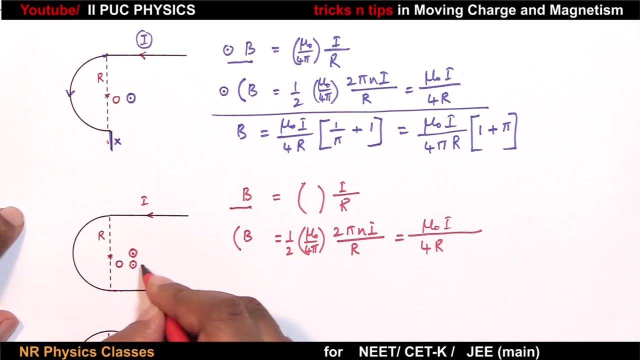 whereas in this case this is along the radius. so field at this point means: because of this conductor, this point is at one end. one end means again this formula now observe directions. because of this stride conductor, magnetic field at this point is outward, perpendicular and outward. because of this stride conduct, also magnetic field is outward. 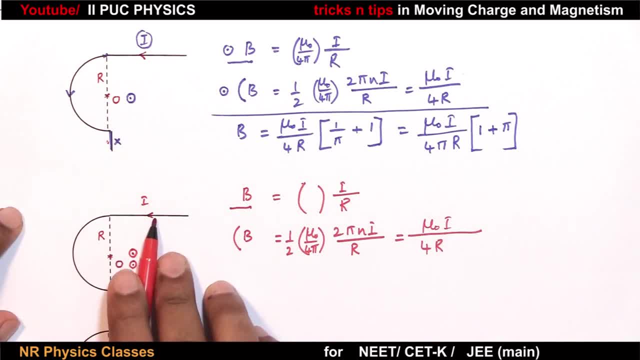 these two magnetic fields are added means field by this plus field by this is two times and field by the arc is also perpendicular and outward. these three magnetic fields are outward. therefore, sum of these two is the resultant. resultant magnetic field is: mu not i by 4 r, mu not i by 4 r, mu not i by 4 r. remaining is 2 by pi plus, remaining is 1. this is the. 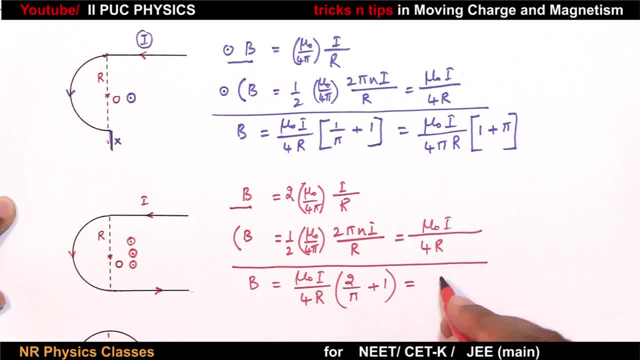 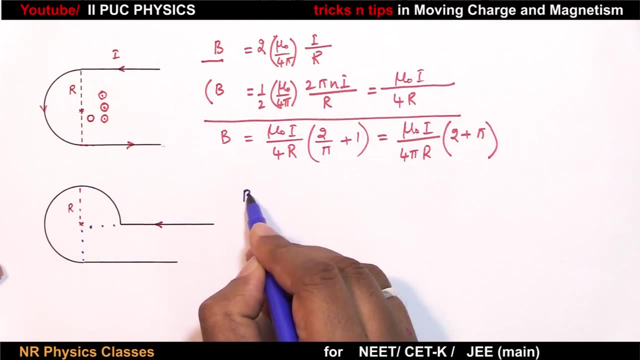 expression. one more form: take pi outside mu, not i, by 4 pi r. pi is outside, means remaining is 2 plus pi. arc subtends an angle 270. magnetic field due to arc is three-fourth. three-fourth is due to 270, three-fourth of constant 2. pi n i by r equal to mu, not by 4 pi 2, pi 1, 2, pi 2, 4, 2. 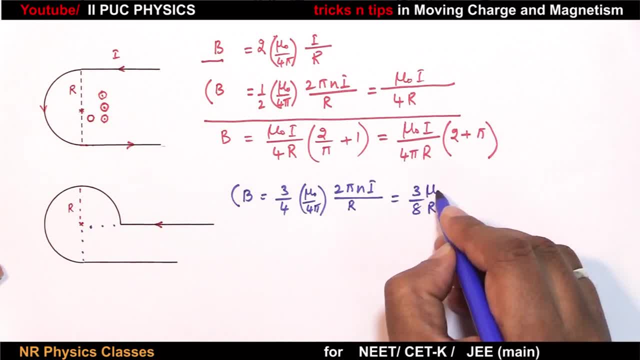 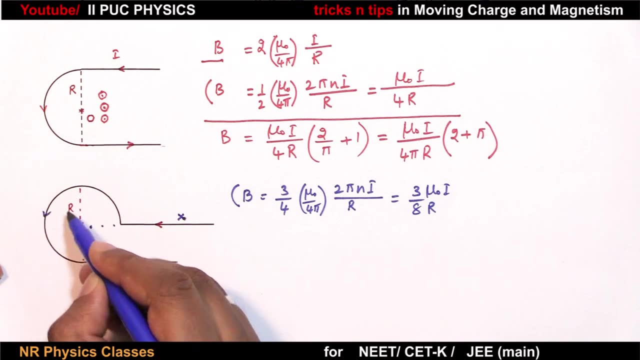 8, 3 by 8 r mu, not i you. this stride conductor is not along the radius, whereas this stride conductor is along the radius. this will not contribute any magnetic field, whereas this stride conductor contributes. this point: o is at one end of the conductor, therefore magnetic field at o due to stride. 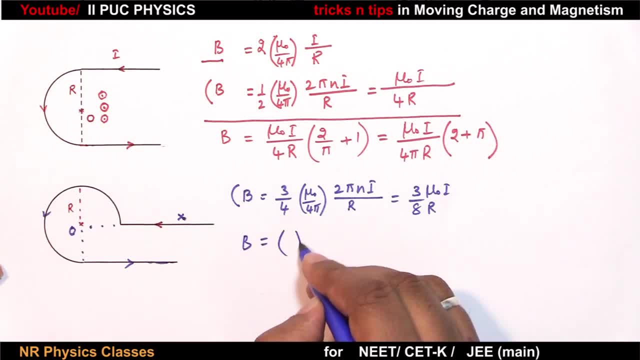 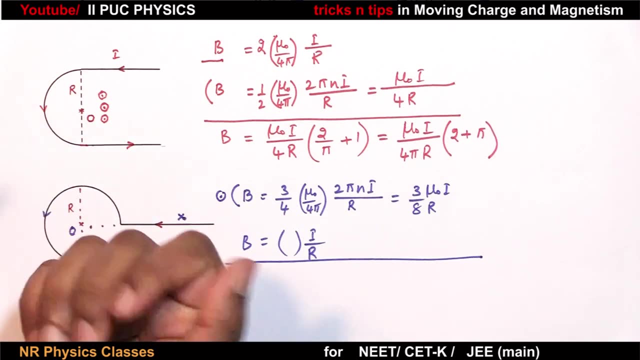 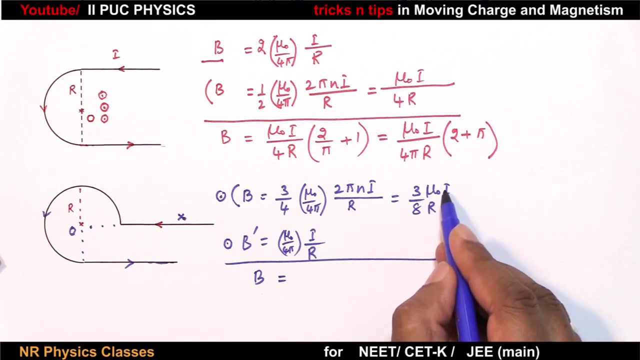 conductor is one end of the stride. conductor is constant i by r. Anticlockwise magnetic field is perpendicular and outward. because of this straight conductor, magnetic field is perpendicular and outward. therefore, resultant of these two means, b equal to this constant, is mu0 I by 4 R, mu0 I by 4 R, mu0 I by 4 R. remaining is three by two. 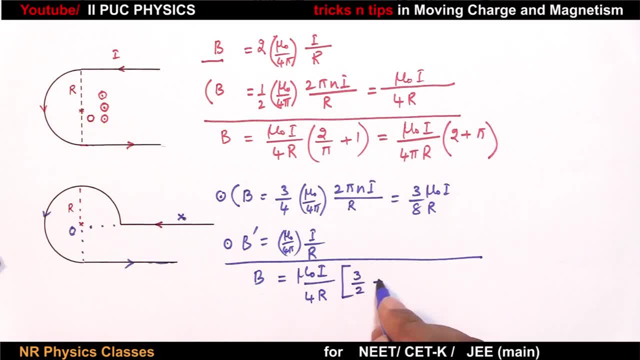 three by two plus one by four. four is outside. why mu not I by four Men? is mu chyba be 9All? of Tamam r. so this is 1 by pi. this is the resultant field, field due to this three-fourth of a circle. 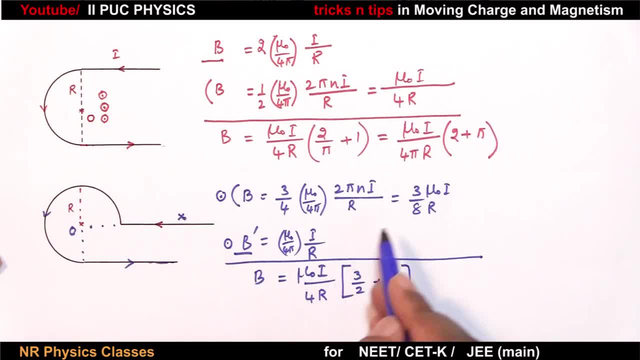 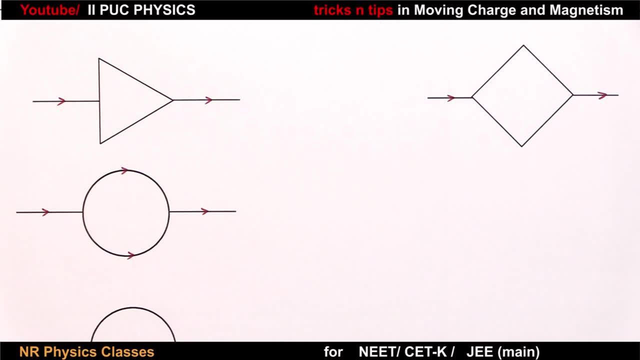 this is field due to straight conductor. therefore, resultant of these two means sum. all these have appeared in examinations. different examinations loop is in the form of a triangle from this conductor current is entering this current branches. this is the outgoing current. what is the magnetic field at the centroid? so this: 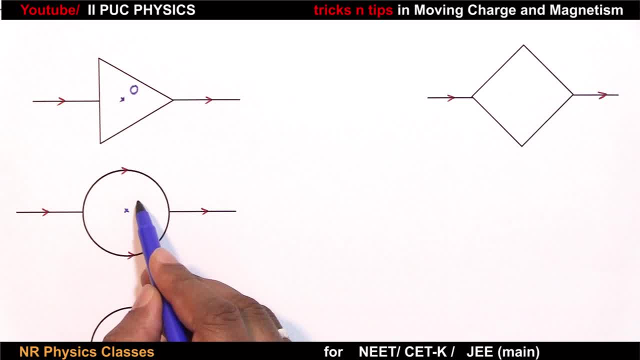 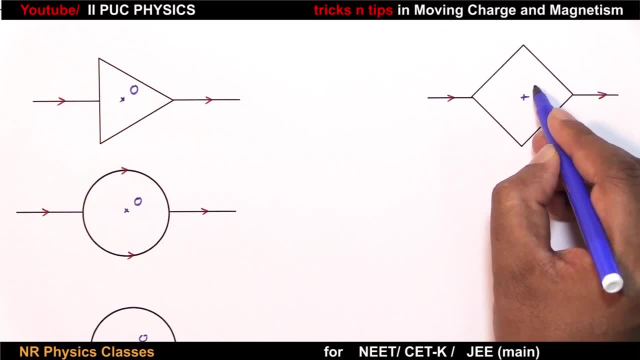 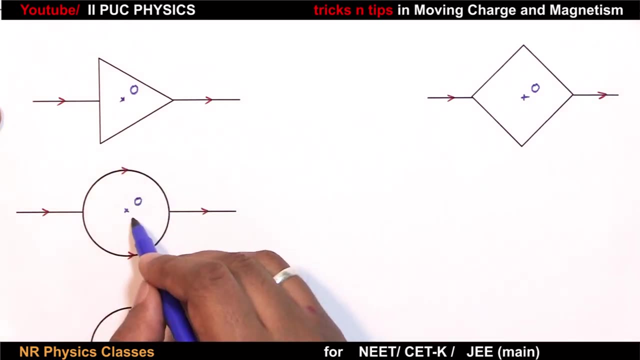 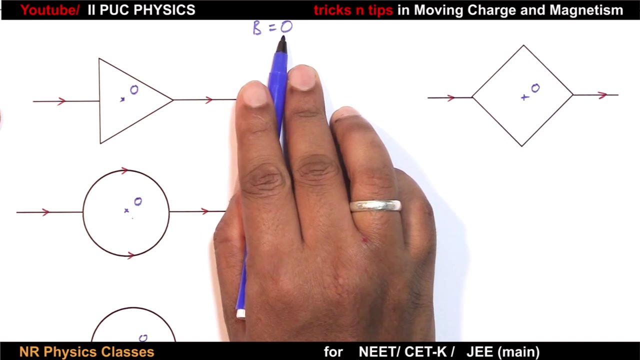 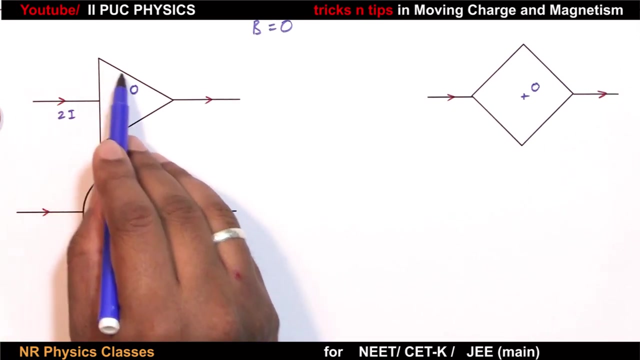 is o. what is the magnetic field at the center? what is the magnetic field at the center? magnetic field at the intersection? okay, if you find such diagrams, magnetic field at the center of such loops is always zero straight away. answer why: magnetic field 0 means assume this current is 2 i, 2 i. this is a conductor. conductor has 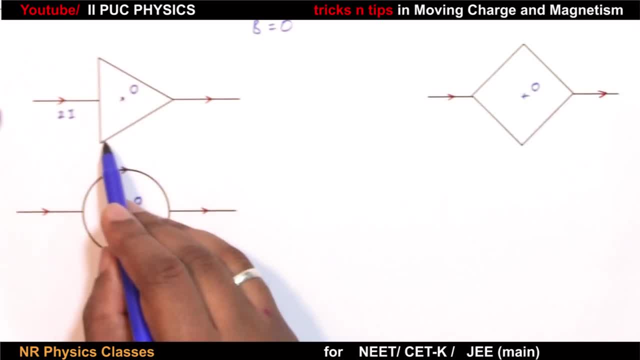 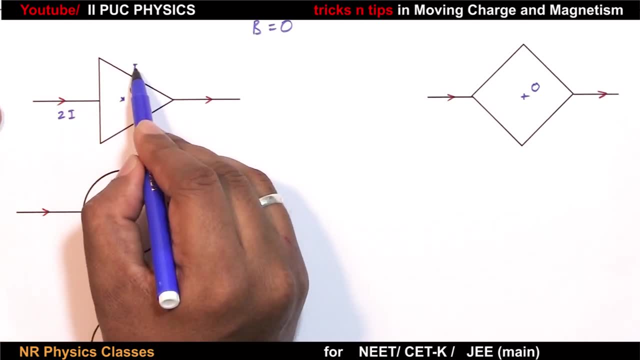 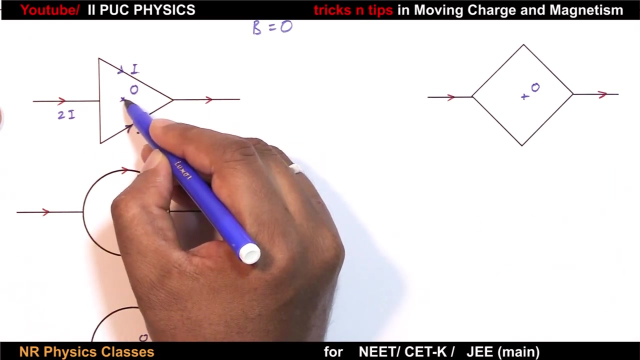 resistance. this length is equal to this. length means resistance of this, equal to resistance of this. therefore, this 2 i splits into i and i. current in the upper half is clockwise like current in the is anti-clockwise, like magnetic field, due to upper half is cancelled by magnetic field due to lower. 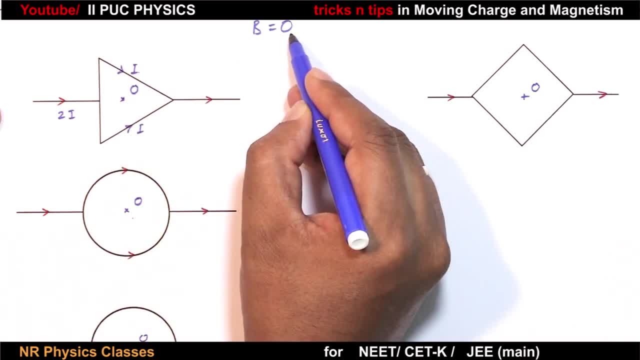 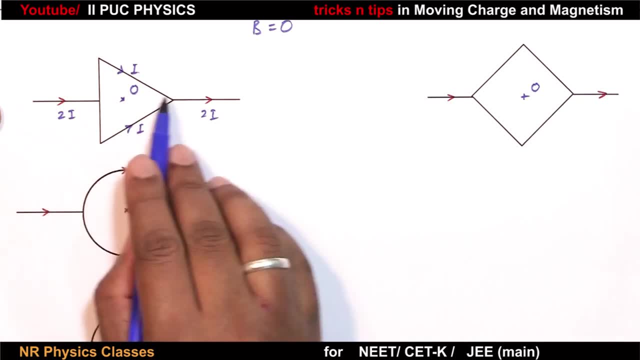 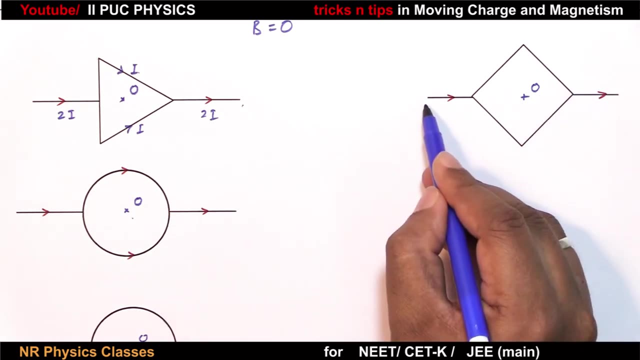 half. that is why resultant field is zero. i and i, according to kirchhoff's current law, becomes 2i. see: current entering the loop is 2i. current leaving the loop is 2i. everything is fine. same thing if this is 2i, this length, equal to this length, equal to this length, equal to this. 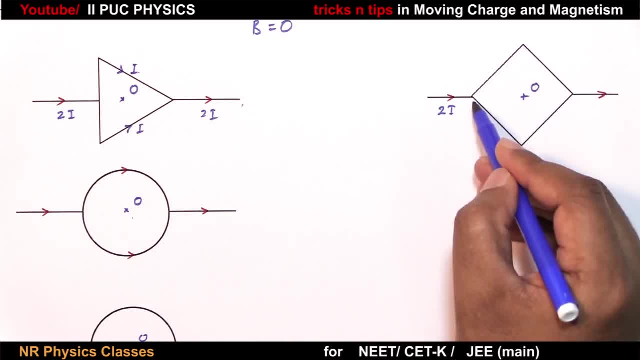 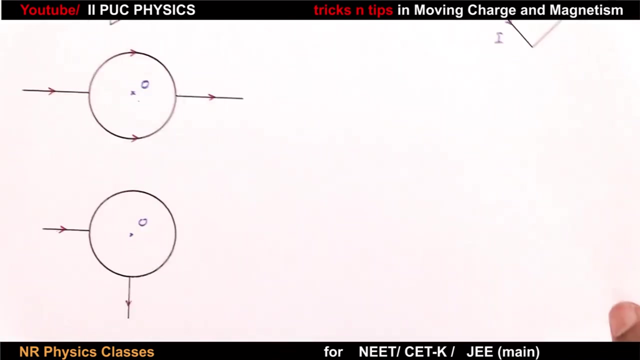 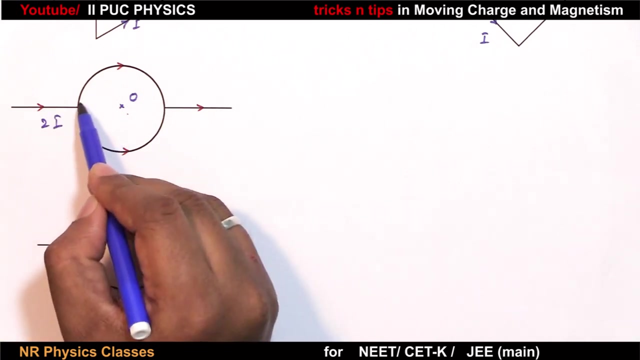 length. so length of upper half is equal to length of lower half. therefore, current through upper half is i, lower half is also i. current magnetic field due to upper half into magnetic field due to lower is out of the loop. therefore resultant magnetic field is zero. now this is 2i, current through upper half, i current through lower half, i. 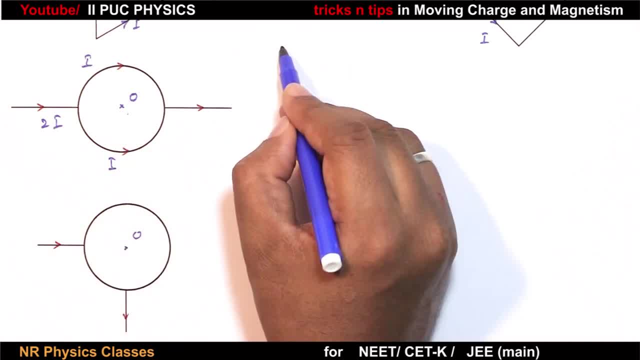 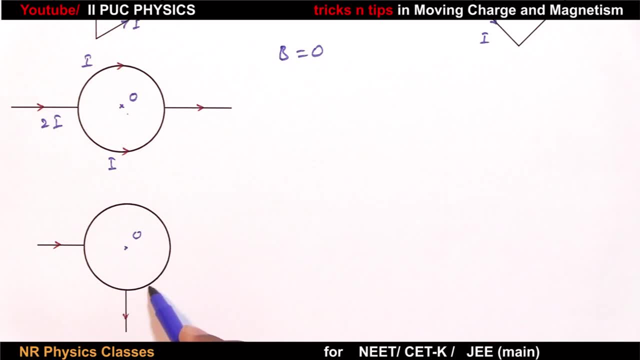 so resultant magnetic field at this entry is zero. come to this: this is three times this length. resistance is proportional to length of the conductor. so resistance of this is three r. resistance of this one-fourth is r three one. for the sake of simplicity, let me take total current as 4i out of 4i. 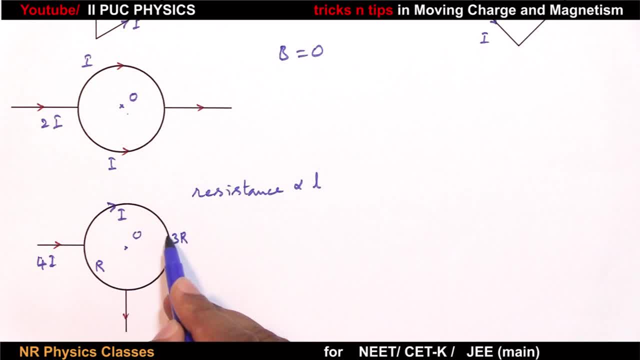 i is the current through three-fourth of a conductor. three i is the current through one-fourth of a conductor, and this diagram is similar to two resistors connected in parallel. this is three-fourth three r. this is one-fourth r. what is the speciality if resistors are connected in parallel? 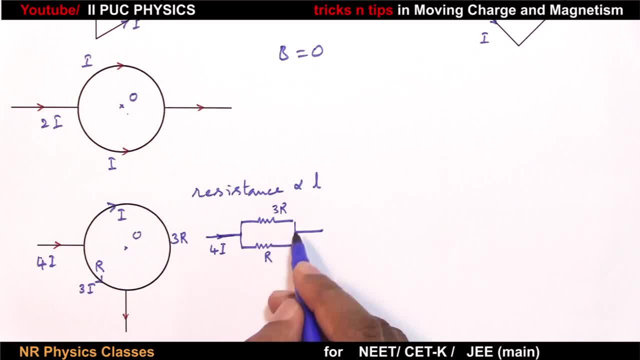 potential difference across them is same. if current through three r is i, current through r is 3 i. so potential difference is product of these two. potential difference is product of these two. these two are equal means. these currents are correct. current distribution is also correct. so magnetic field at the center, due to upper half of three times the length, lower half of one time. 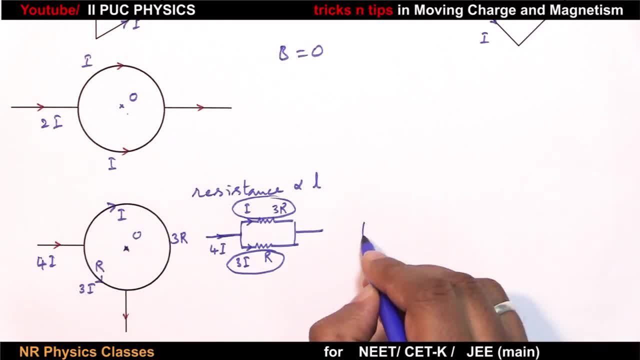 the length those two magnetic differences are corresponding, then the resultant match that length be equal less. therefore we can infer that current through air vector vector distribution is also equal to star hyperère creating. the fields are equal and opposite, therefore resultant field equal to zero. all the four diagrams have 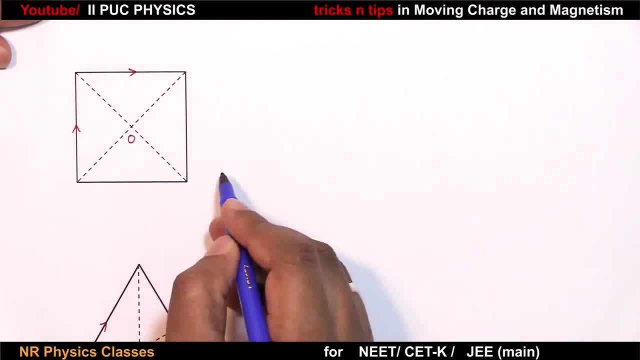 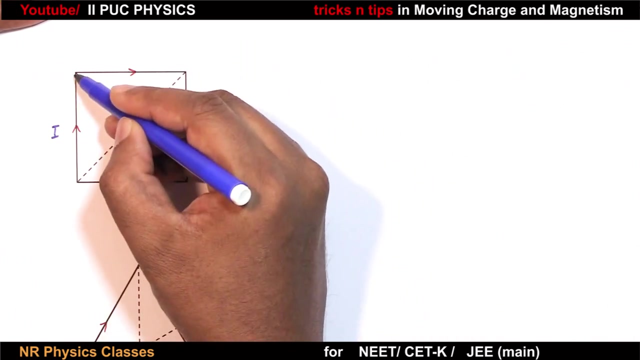 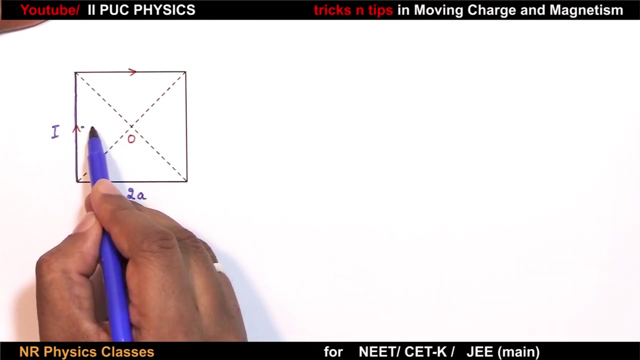 appeared in different exams. now, instead of arc or circle, what if it is in the form of square triangle? okay, now let this be a square of length, 2a for time being. 2a current through the conductor. is i consider this straight conductor? for this straight conductor, point o. this is the shortest. 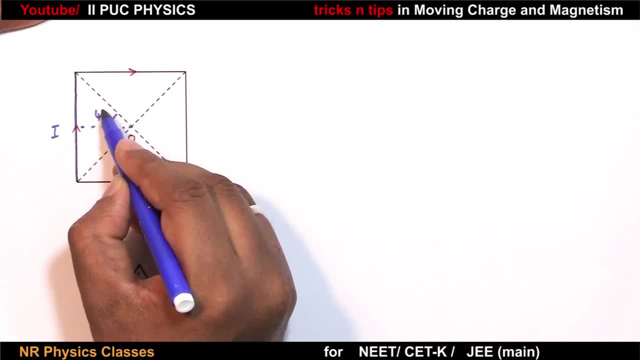 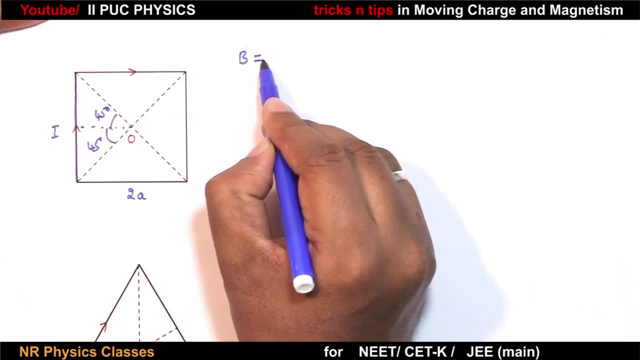 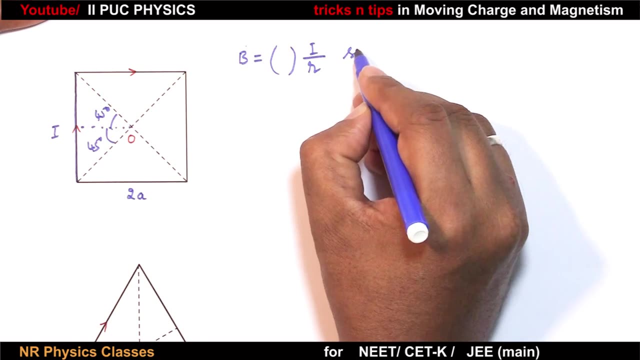 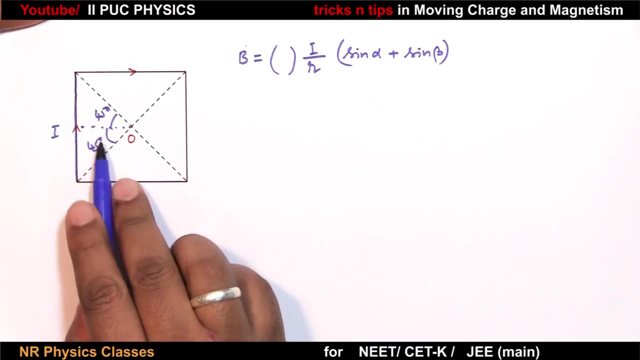 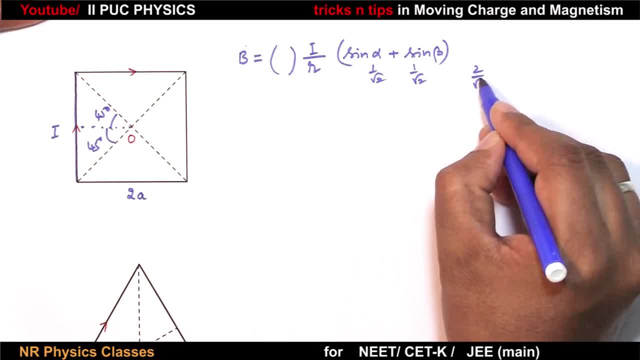 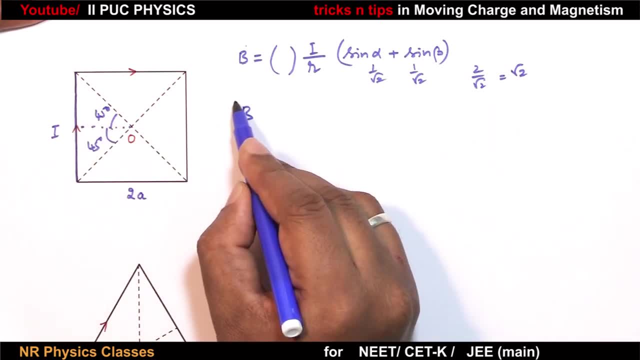 1 by root 2, 1 by root 2 plus 1 by root 2 is 2 by root 2. 2 by root 2 is root 2.. therefore, magnetic field due to this conductor, this straight conductor, is equal to constant, is mu. 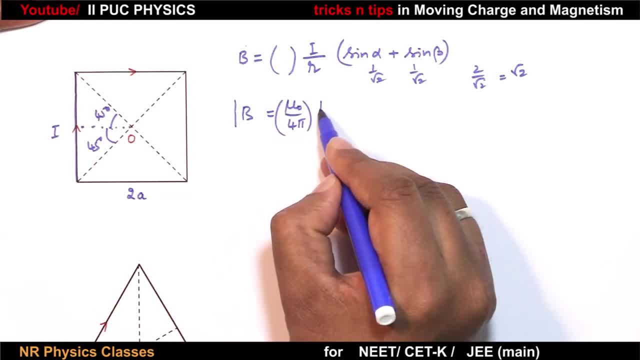 0 by 4 pi, current by r, is distance between these two. if total distance is 2a, then half of the distance is a. therefore this distance is a. a sine alpha plus sine beta, sine 45 plus sine 45 is root 2, root 2. 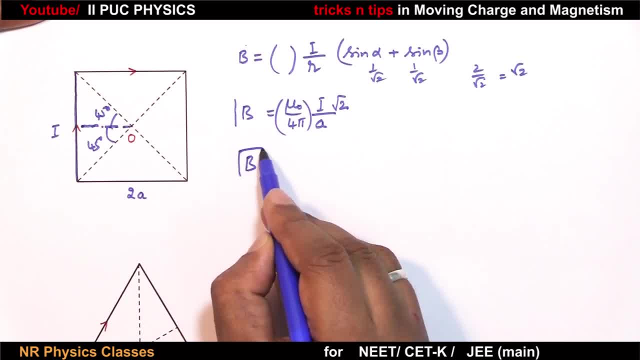 now magnetic field at o due to entire square. there are four sides. therefore 4 times mu, 0 by 4 pi, 4 times 4 root, 2 i by a. this is the magnetic field. if direction of current is clockwise, then magnetic field is into this, magnetic field is into the plane. 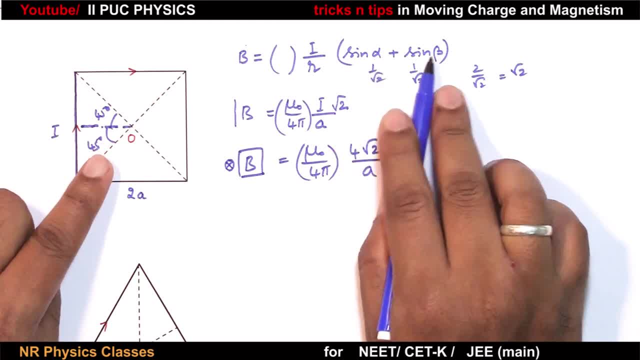 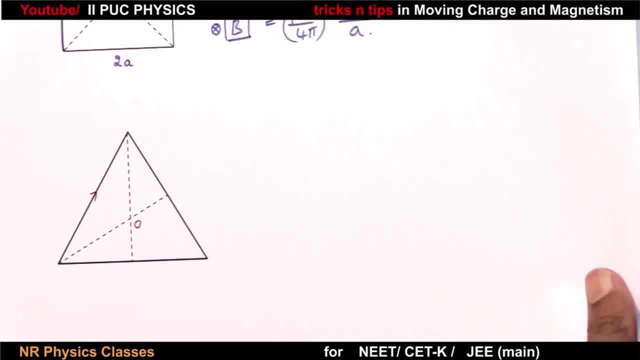 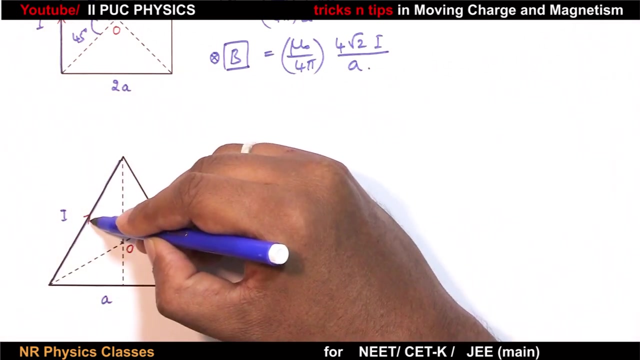 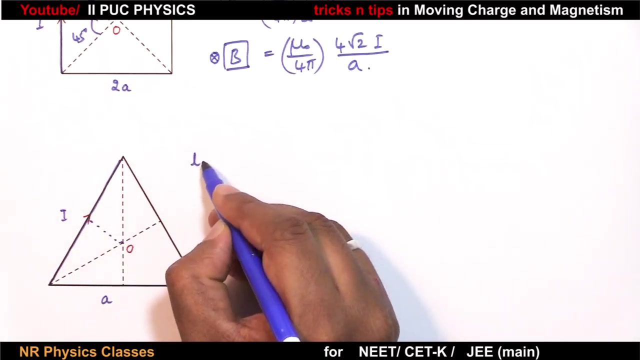 use this equation: substitute 45, 45, simplifying, so multiplied by 4. now this is centroid current is. I let length of each side be a. consider this part of the conductor, from this conductor to point O, shortest distance. this shortest distance, let it be L: L. this angle is 60 degree. this angle is also 60 degree. 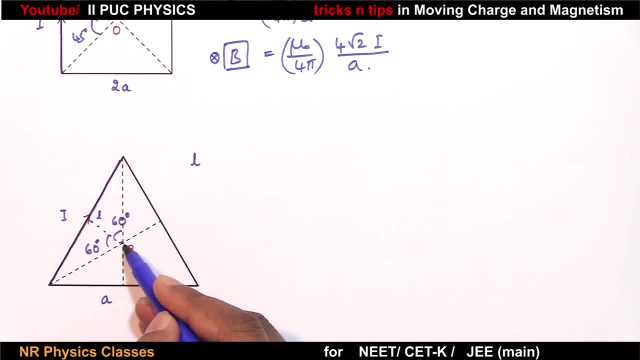 straight conductor field at some point. magnetic field equal to constant I by R, sine alpha plus sine beta, sine 60 plus sine 60 s. root 3 by 2 plus root 3 by 2, equal to root 3. therefore, magnetic field due to one side is constant I by R into. 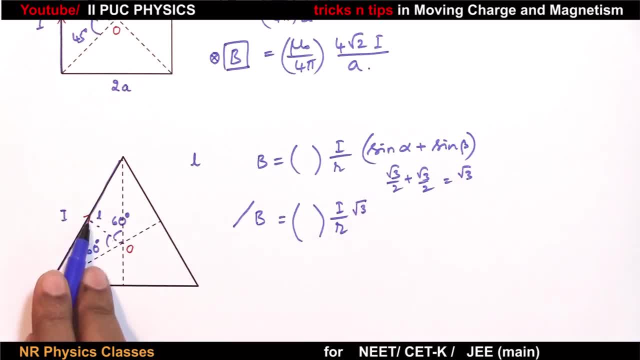 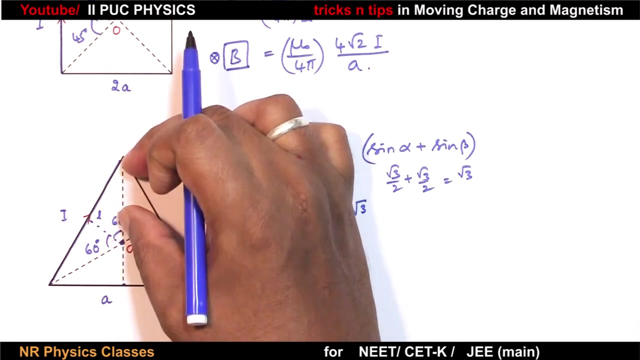 root 3, now L. what we want is the shortest distance, L. okay. so distance of the centroid from one side of the conductor means L equal to length of each side is a minute. are all diameters given as 1 by my plus 1, 1 North? did we? 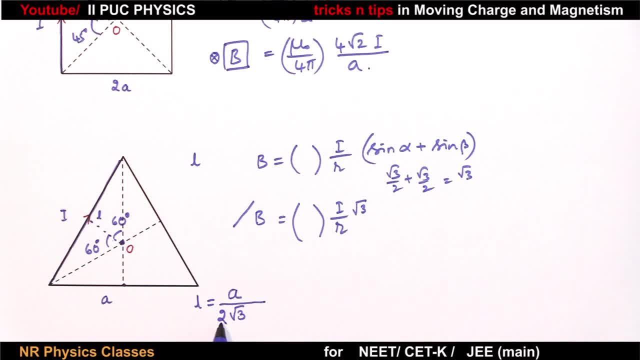 put about that I mistakenly did, why I misездem, pictured in orange in white. this is that this red triangle write and then X P 1, half of L length is equal to 20 plus R. minus X P 2, half your получилось. I will r E to myself minus X P 2 plus R over R minus X. calm is an the constant R Zeit. 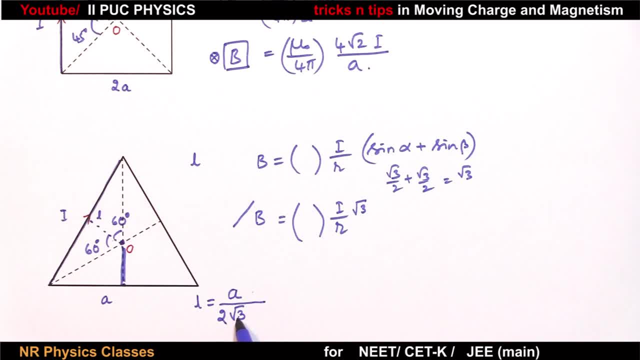 capitalajik gained by the hayat pueden D communications by không ben jeder length into 1 by root 3. okay, so this a becomes a by 2 root 3, equal to constant mu naught by 4 pi. this root 3 goes to numerator root 3 into root 3 is 3, 2 into 3 is 6, 6, i by a, 6, i by a. therefore,